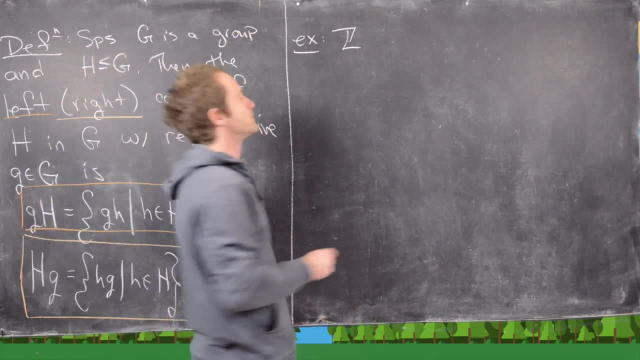 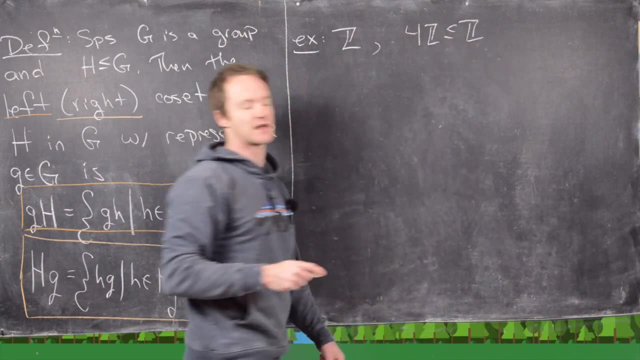 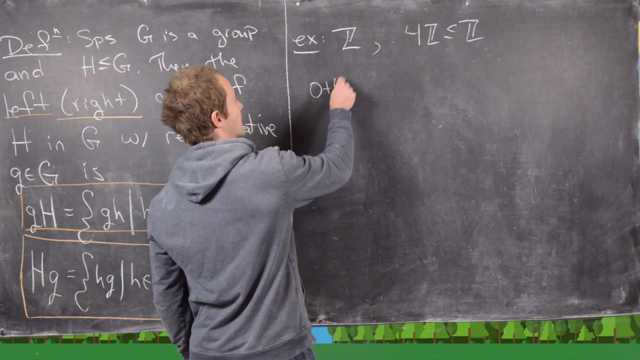 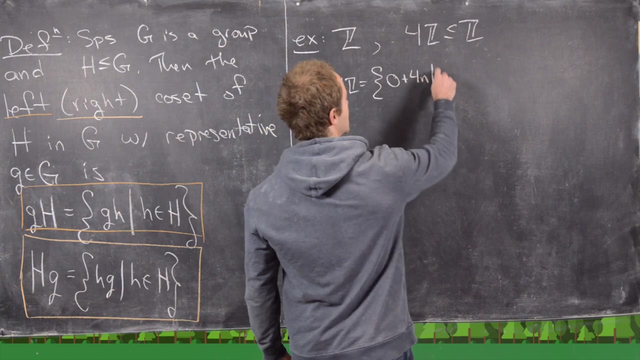 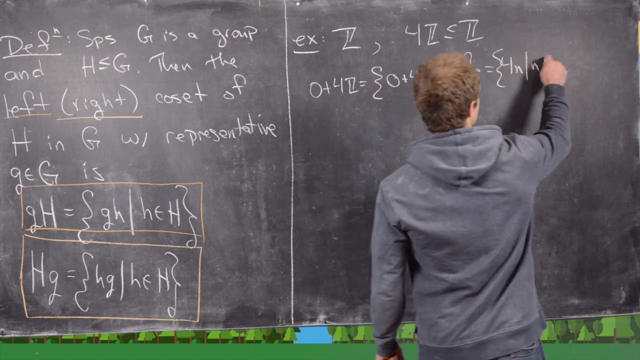 So let's say our group is Z and then let's say our subgroup is 4Z. So in a previous video we proved that all subgroups of Z are of the form NZ. So here let's take 4Z and now let's look at 0 plus 4Z. And so what this is going to be equal to is 0 plus 4N as N runs through all of Z. In other words this is just equal to 4N as N runs through all of Z or just 4Z itself. So this is equal to 4N as N runs through all of Z. So this is equal to 4N as N runs through all of Z. So this is equal to 4N as N runs through all of Z. 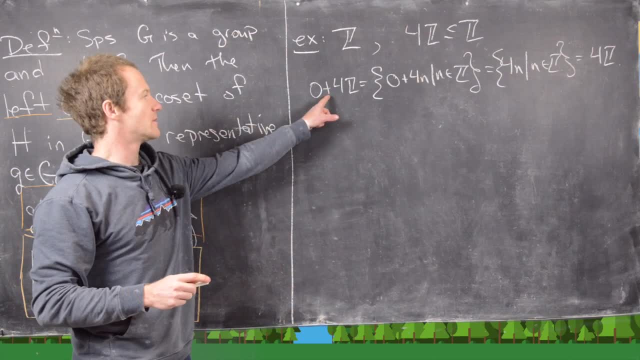 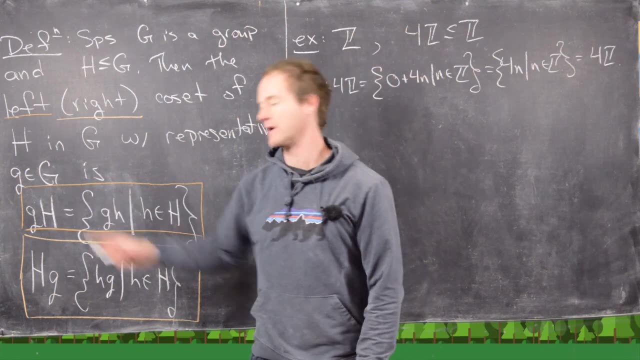 So that's the coset of 0. And notice here I've used plus because we're in an additive group here. But in general if you don't know the operation for the group you just kind of put them next to 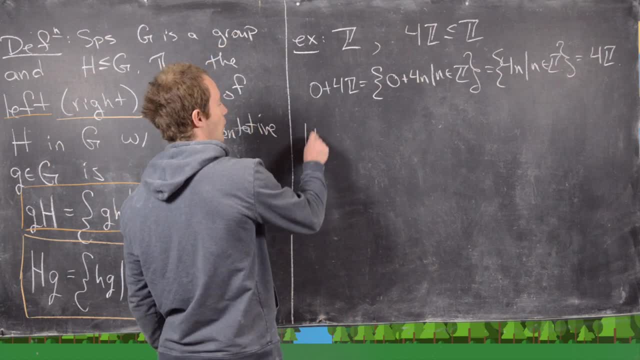 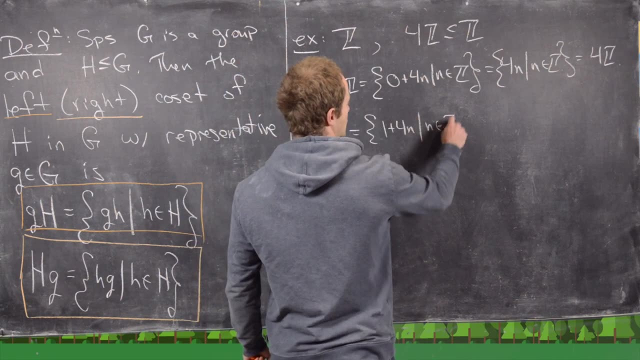 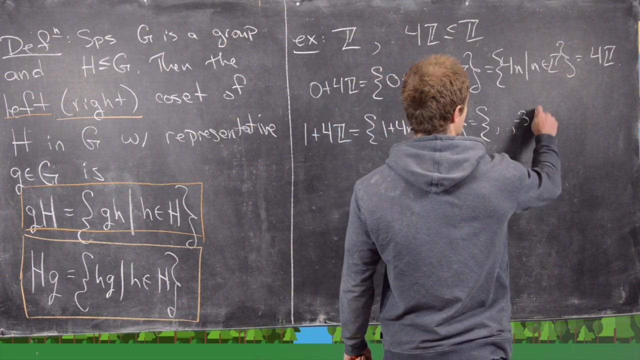 each other like this. Okay so now let's look at 1 plus 4Z. So this is everything of the form 1 plus 4N where N runs from all of Z. So in other words this is like the numbers minus 3, 1, 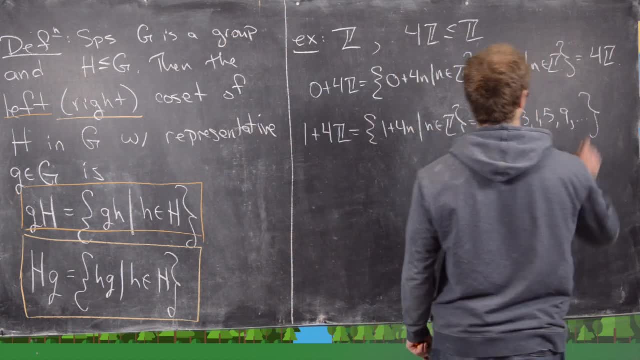 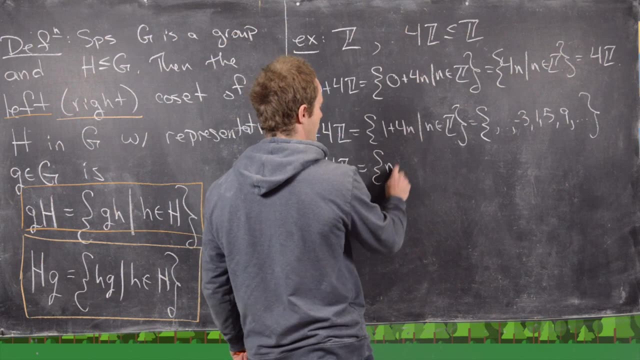 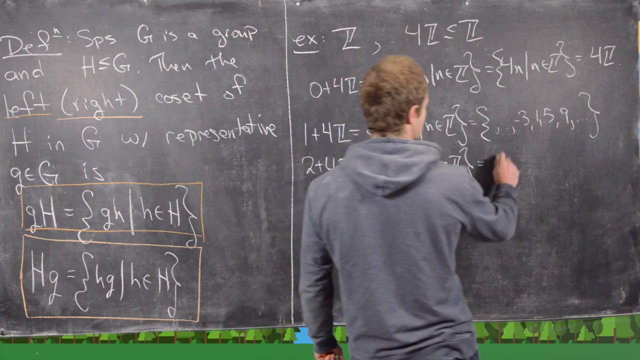 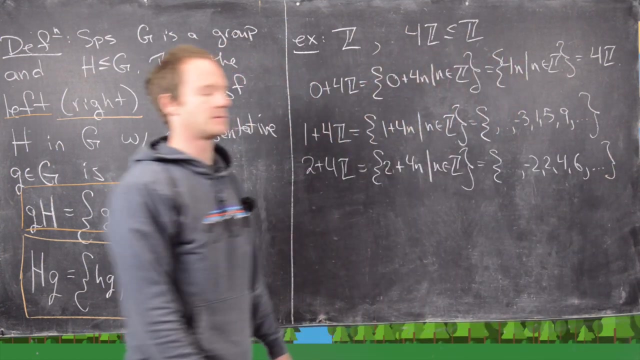 5, 9, and so on and so forth. Great. Now let's look at 2 plus 4Z. So this will be everything of the form 2 plus 4N where N runs from all of the elements in Z. So this is going to be like minus 2, 2, 4, 6, and so on and so forth. Great. And then one more. Let's do 3 plus 4Z. 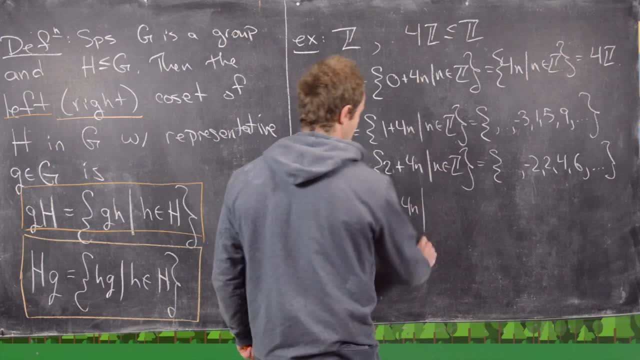 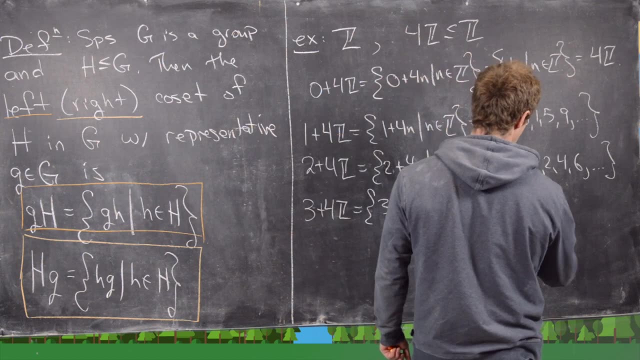 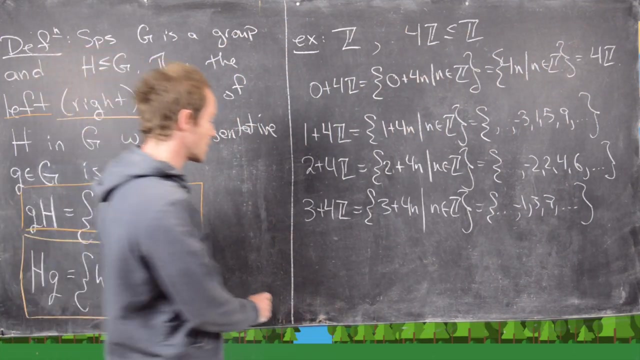 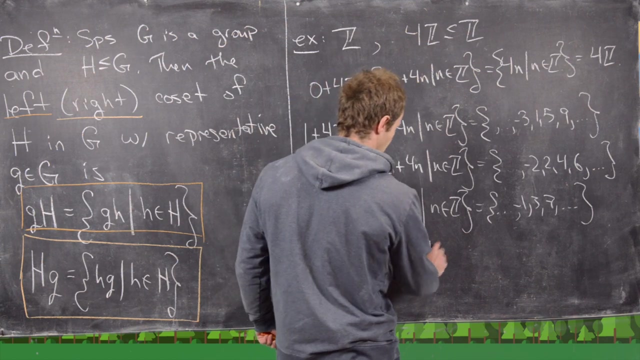 So this is going to be equal to 3 plus 4N where N runs through all of the elements from Z. So this is going to be like minus 1, 3, let's see 7, and so on and so forth. And now notice if we go to 4 plus 4Z we're going to get 4 plus 4N where N runs through all of Z. But notice we can just re-index how this set is going to be. So we're going to get 4 plus 4N where N runs through all of Z. 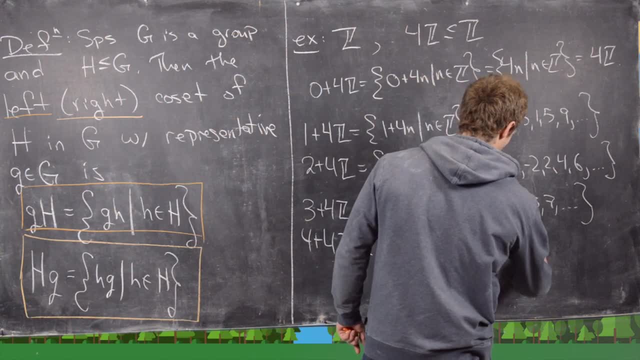 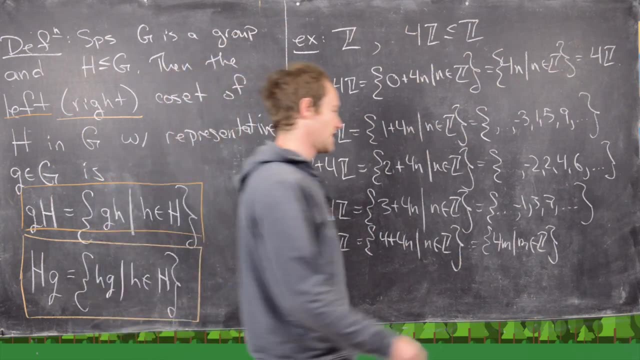 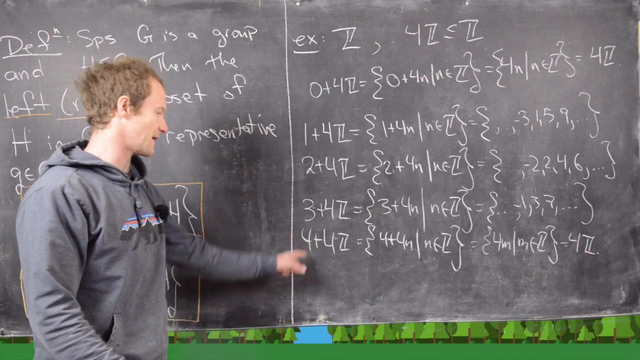 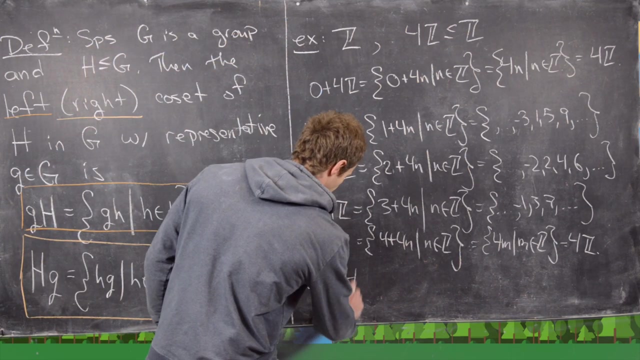 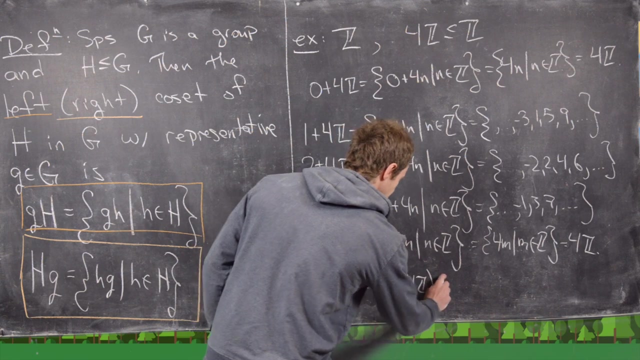 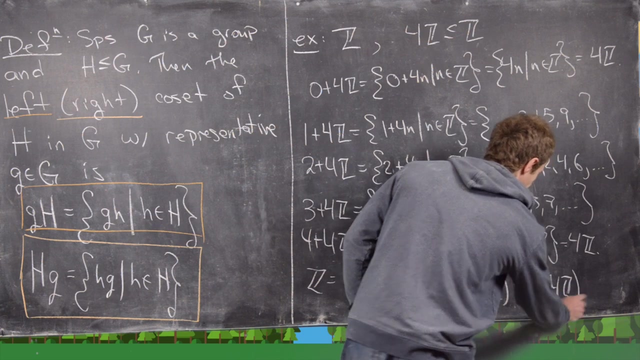 And that's going to give us 4M where M runs through all of Z. If we absorb the 4 into the 4 times N and then this is just going to give us 4Z exactly. So we're back at what we started with. So 0 plus 4Z is the same thing as 4 plus 4Z. In fact I think it's pretty easy to see that the integers decompose into this disjoint union 1 plus 4Z, 2 plus 4Z, and 3 plus 4Z. And in fact this kind of property will prove carefully later. 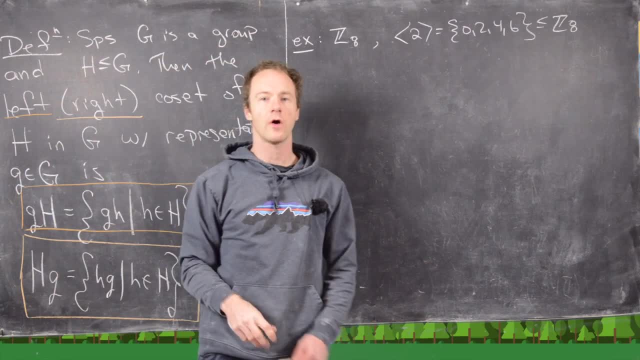 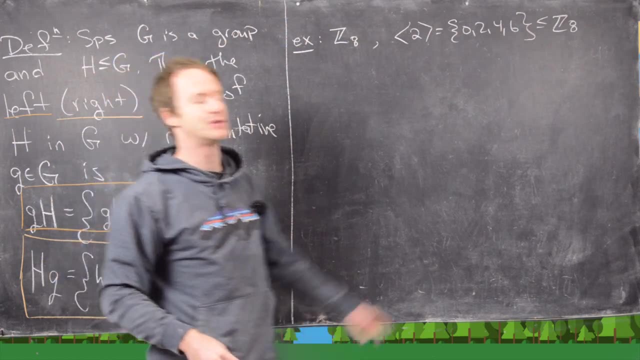 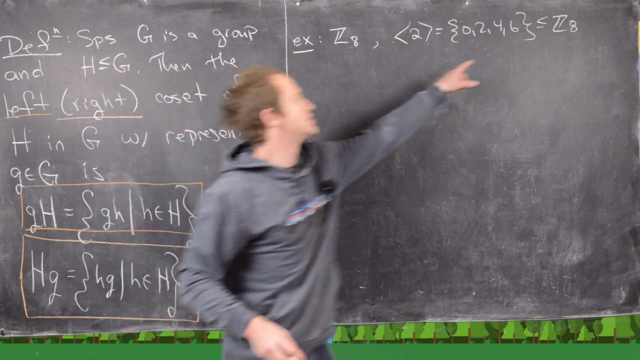 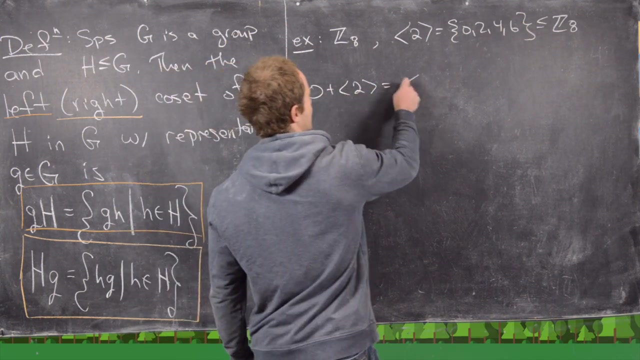 All right I'll clean up the board and we'll look at another example. Okay so for our next example for the group I want to look at Z8 and then I want to look at the cyclic subgroup generated by 2. So that's going to give us 0, 2, 4, and 6. And recall here our addition is modulo 8. So if I do 2 times 6 I get 8 which is 0 obviously. Okay so now let's look 0 plus this cyclic subgroup is obviously going to be this cyclic subgroup because all we've done is added 0 to every element here. 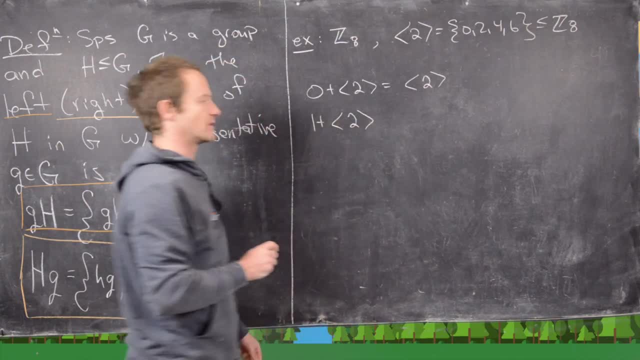 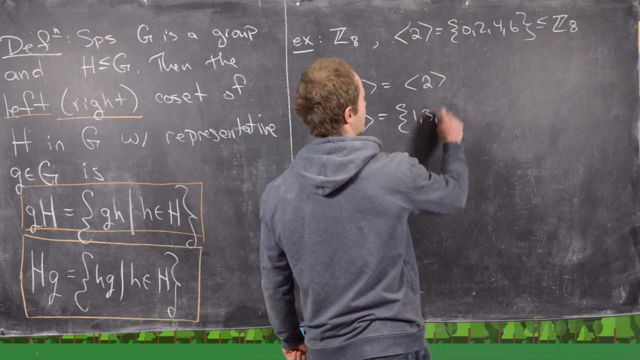 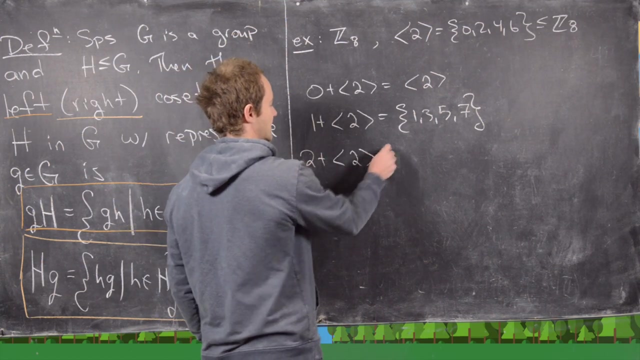 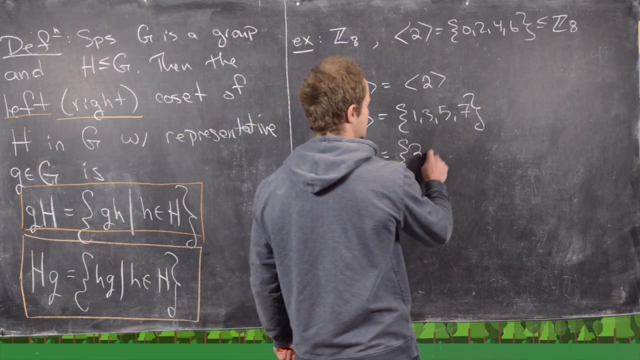 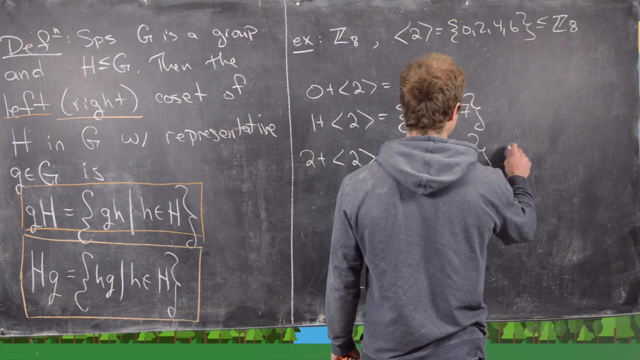 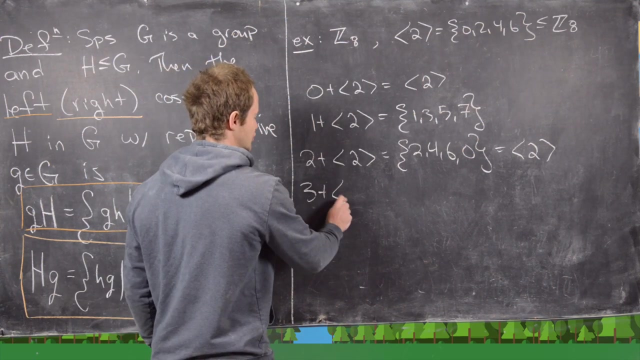 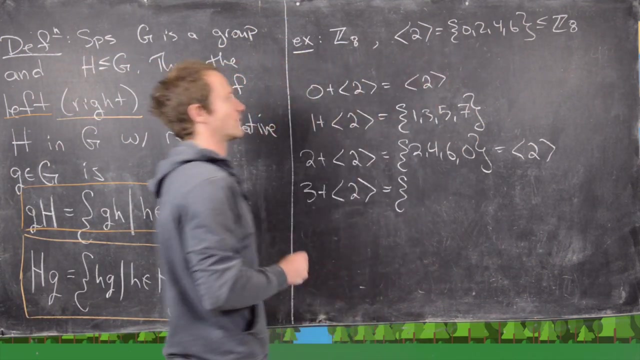 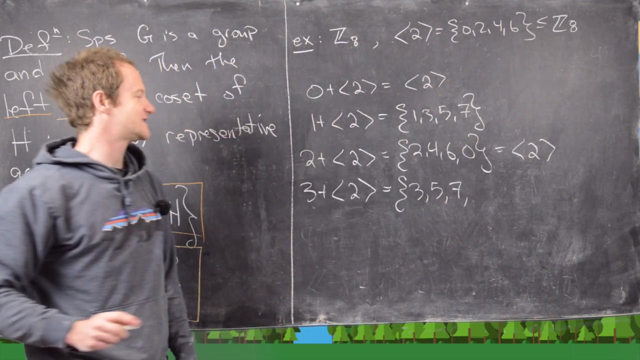 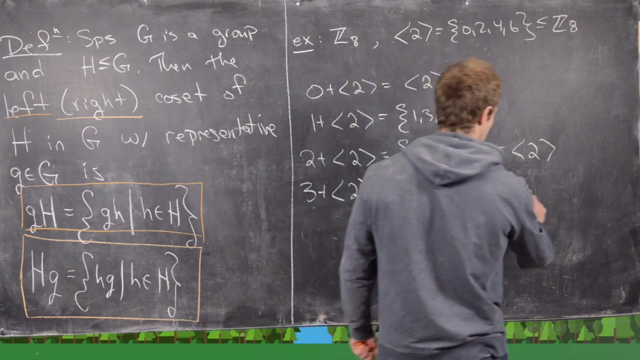 Now let's do 1 plus this cyclic subgroup. So in other words we're going to add 1 to every element of this subgroup. So we're going to get 1, 3, 5, and 7. Great. Now let's do 2 plus this cyclic subgroup. So in other words we're going to write we're going to add 2 to every element from this subgroup. So that's going to give us 2, 4, 6. And then 6 plus 2 is 8 but that's back at 0. And notice that's exactly what we started with which was the cyclic subgroup itself. Now I think we can probably see what's going on but let's just check with one more case. Let's do 3 plus the cyclic subgroup. So we're going to add 3 to every element of this subgroup. So that'll give us 3, 5, 7. And then we have 6 plus 3 which is 9. But 9 is the same thing as 1 mod 8. So that gives us the same thing as 1 plus the cyclic subgroup generated by 2. 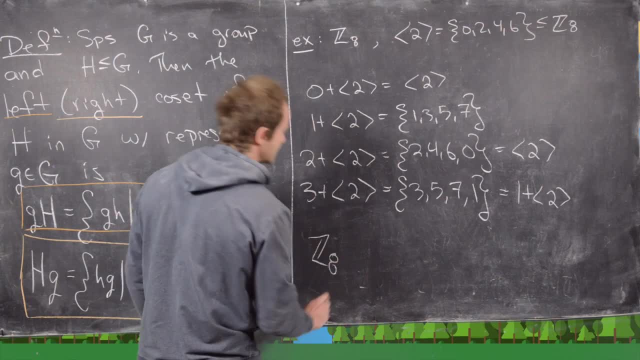 So I think we can see again that z8 is going to decompose as follows. So this is the cyclic subgroup generated by 2. 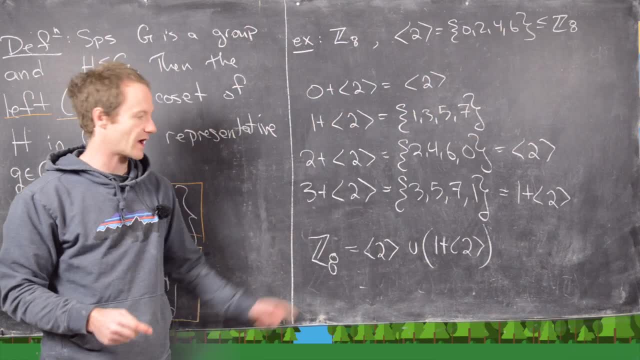 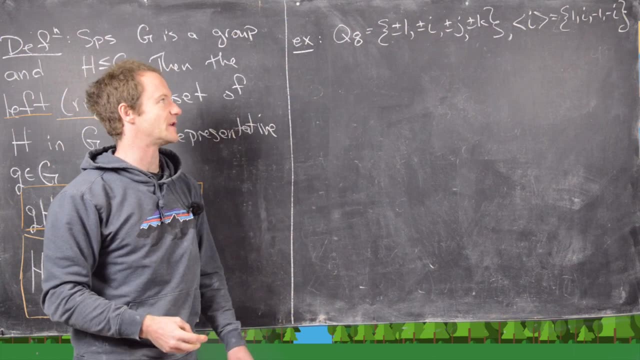 This coset with representative 1. Okay great. I'll clean up the board and then we'll look at another example. Okay so the group in the next example I'll take to be the quaternions. 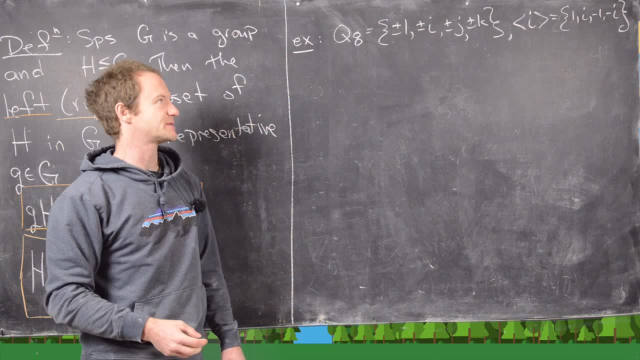 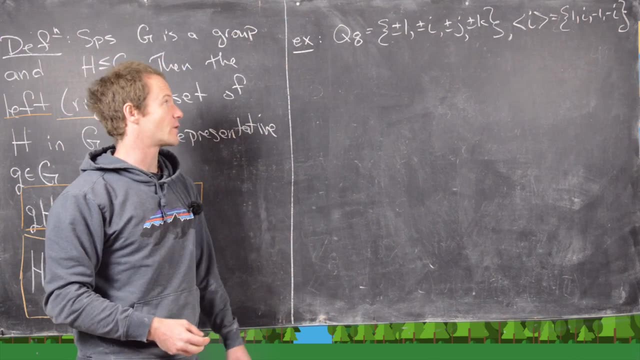 So recall that's a non-abelian group of order 8. I've got plus minus 1 plus minus i plus minus j and plus minus k. I've got a video on the quaternions if you need to review that. But we know that i squared equals j squared equals k squared is negative 1 and then i times j is k and then there are some other properties as well. 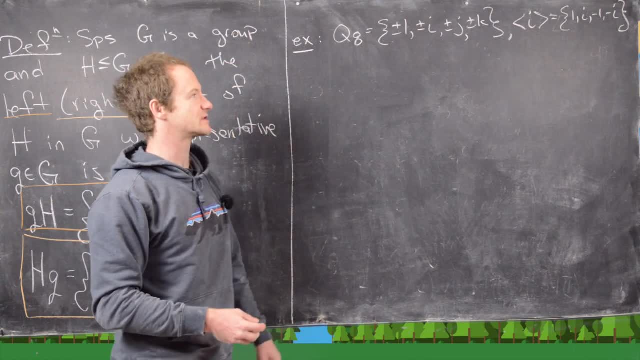 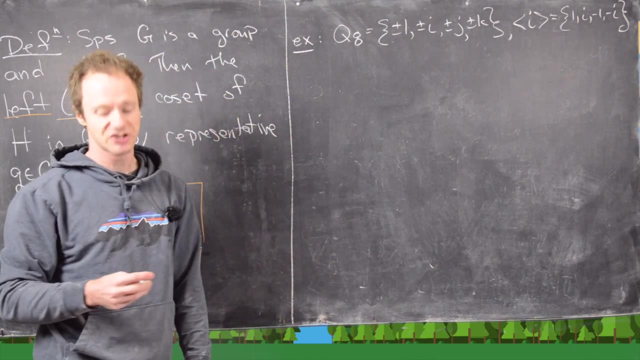 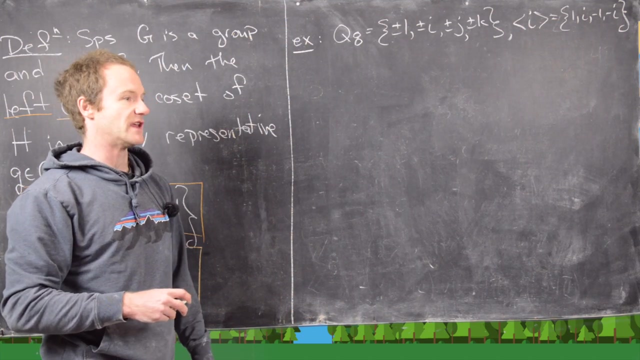 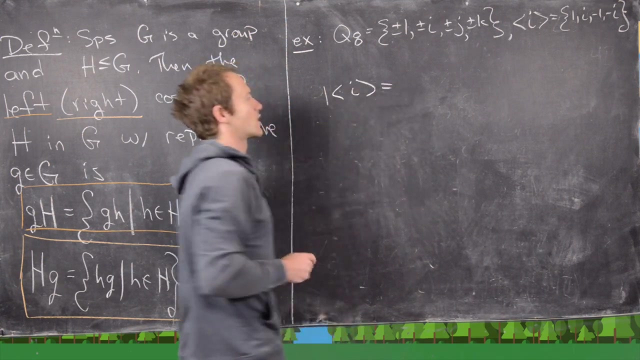 So we'll take the cyclic subgroup generated by i. So that's going to give us 1 i minus 1 and minus i. So it's a group of order 4. Okay so now here our multiplication is our operation. So we won't have this plus as we're defining the coset but we'll just have multiplication. So we'll have the coset with representative the identity. So in other words we're going to multiply every element of this i by 1. So notice that's just going to give us 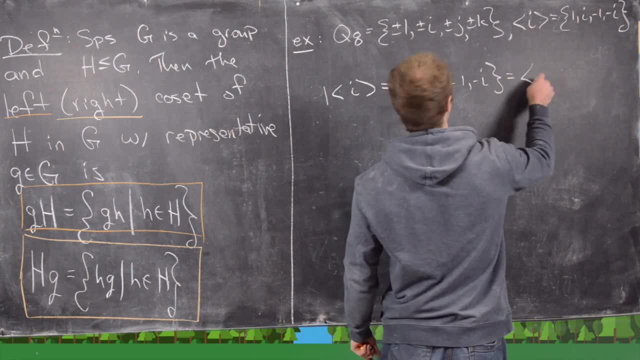 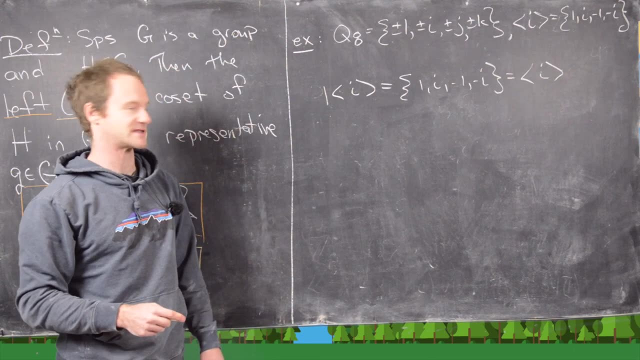 1 i minus 1 minus i. That gives us exactly what we started with. In fact the coset with representative identity is always just going to be that subgroup. Okay so now let's take an element 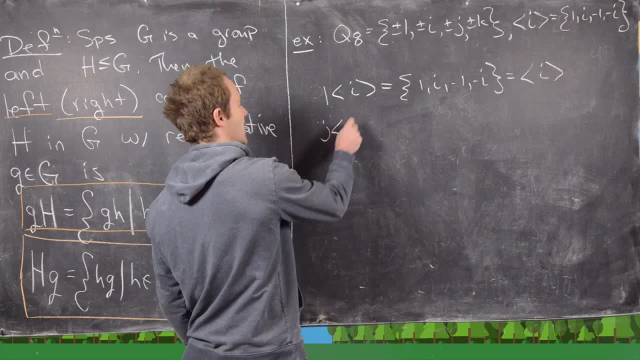 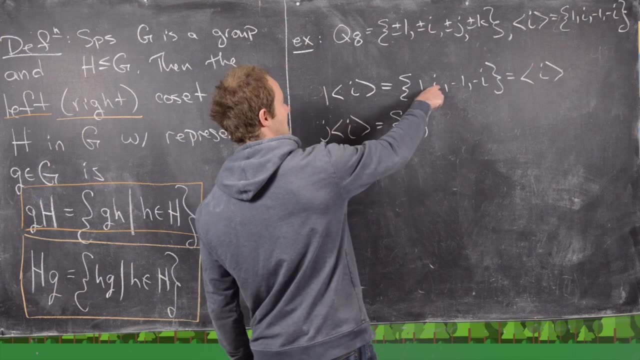 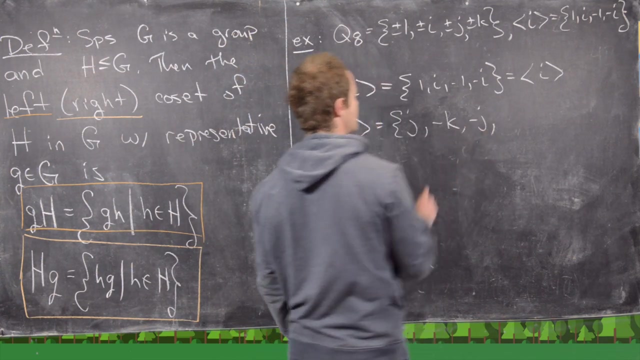 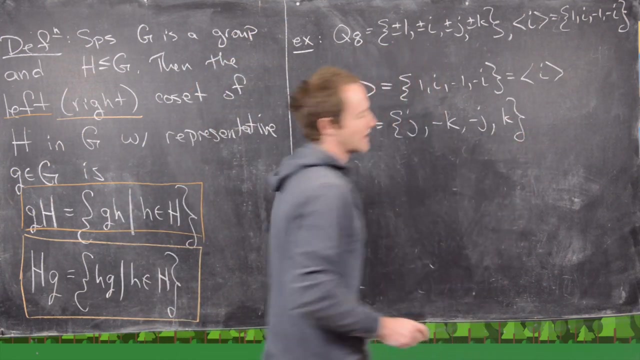 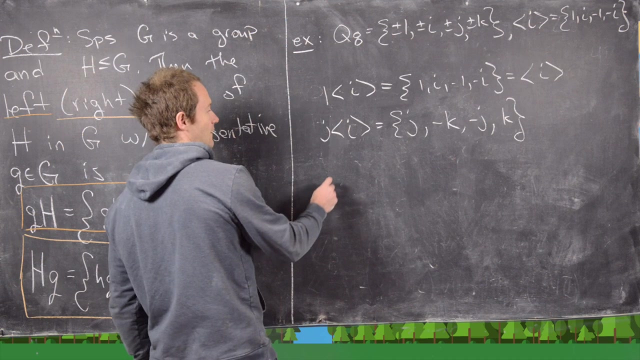 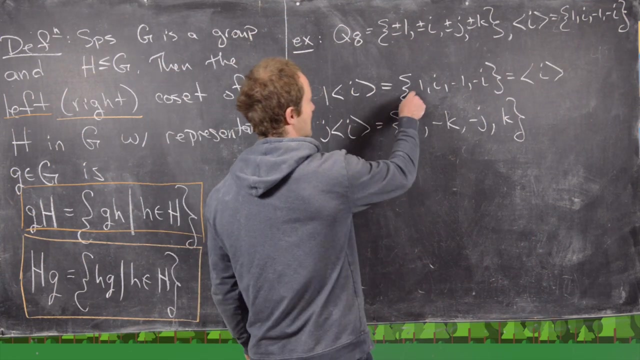 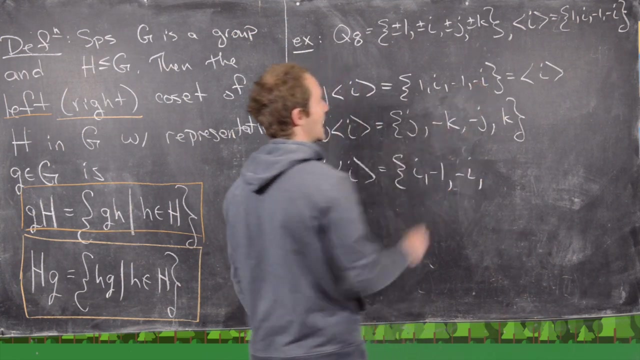 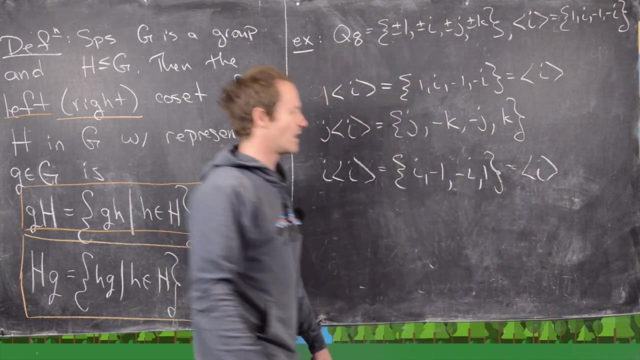 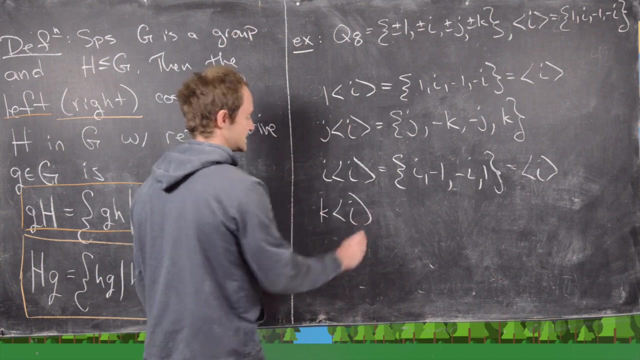 maybe outside of the subgroup. Let's take j multiplied by every element in this subgroup. So notice that's going to give us j. j times i is negative k and then j times negative 1 is negative j. And then again j times i is negative k but we have another minus sign there so that gives us k. So again here we're using quite a bit from the structure of the quaternions. So check out that other video if you need to. Okay now let's do maybe i coset i. So let's see that's going to give us we're going to multiply everything in the subgroup by i. So that'll give us i negative 1 negative i and then i times i minus i. So that's going to give us i minus 1 minus i. So that's going to give us i is i squared which is negative 1 and then we have another minus sign which gives us 1. So notice that's just the cyclic subgroup we started with. So let's do one more although maybe it's kind of clear what's going on here. Let's do the coset with representative k. 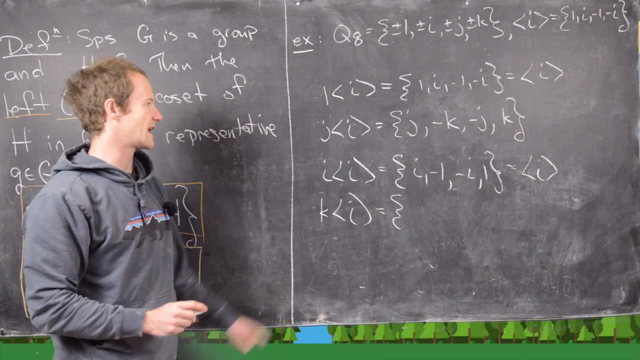 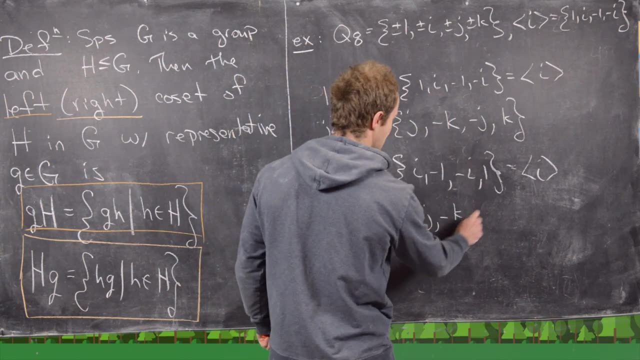 So that means we need to multiply everything in this subgroup by k. We have k times 1 is k. k times i is j. k times negative 1 is negative k and then here we have negative j. Great. 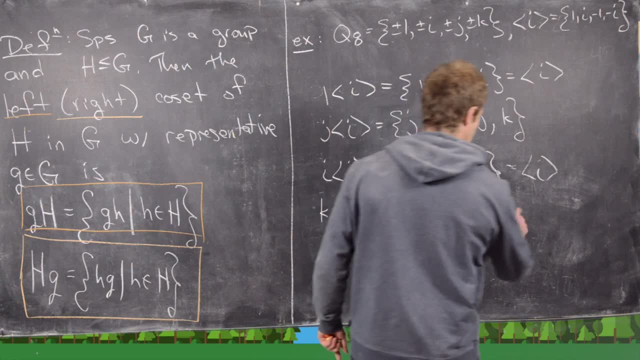 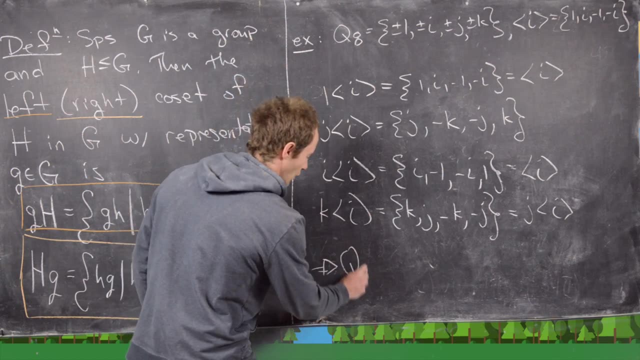 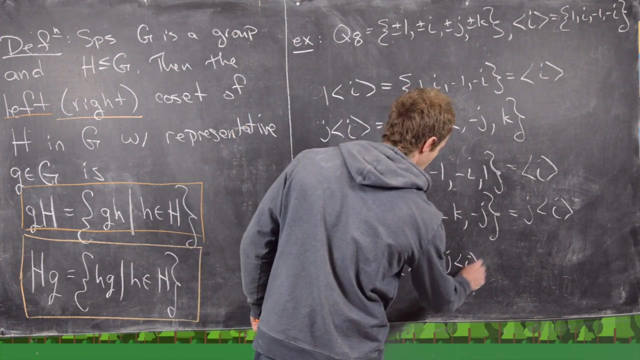 But now notice that's exactly the same thing as this coset. So we get j i. Okay good and now notice here we have the quaternions are breaking up into this cyclic subgroup and the coset with we've got a couple of choices for the representative. Let's just choose this one j. Okay good. So I've got a 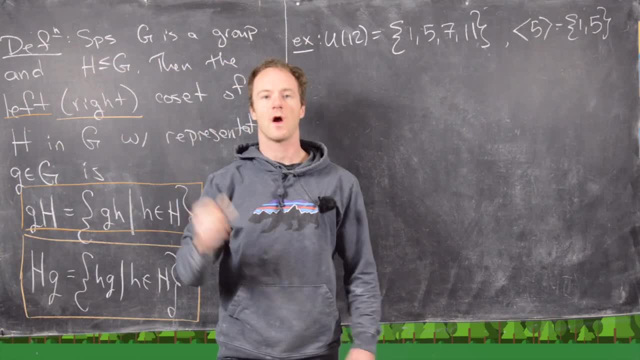 couple more examples I want to do before the end of this video. Okay so for our next example I want to look at the group of units. I'm going to look at the group of units. I'm going to look at the 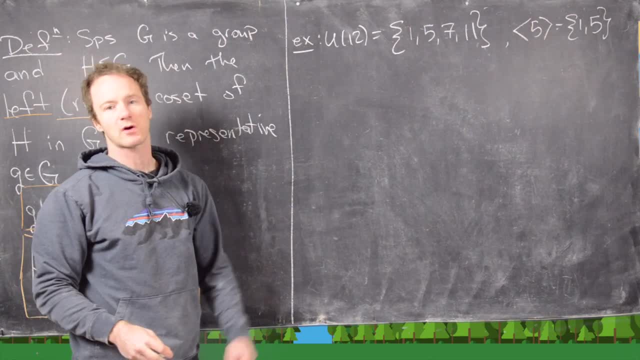 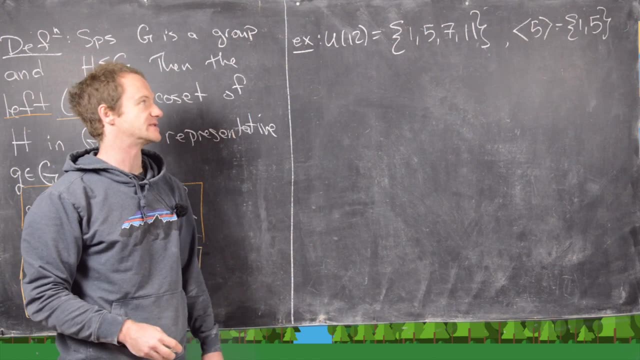 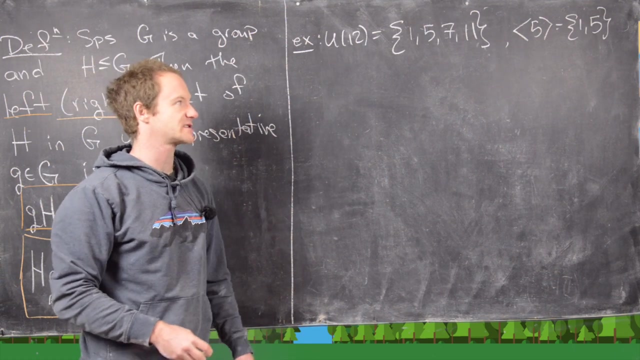 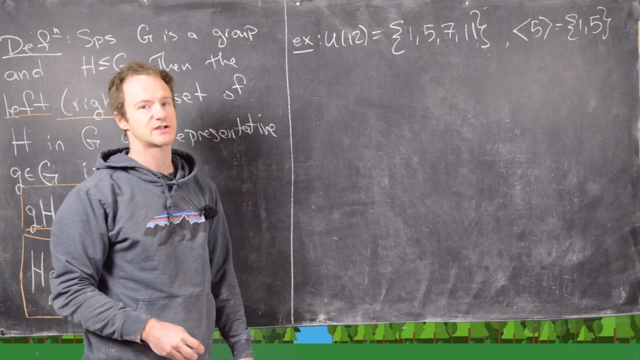 modulo 12. In other words u12 and recall that is everything between 1 and 12 that's relatively prime to 12 and then our operation is multiplication modulo 12. So all we're left with is 1 5 7 and 11 and then let's take the cyclic subgroup generated by 5 and so notice that just gives us 1 and 5 and that's because 5 squared is 25 which is 1 mod 12. Now let's look at the cosets. So notice the coset is 1 and 5 and that's because 5 squared is 25 which is 1 mod 12. Now let's look at the cosets. 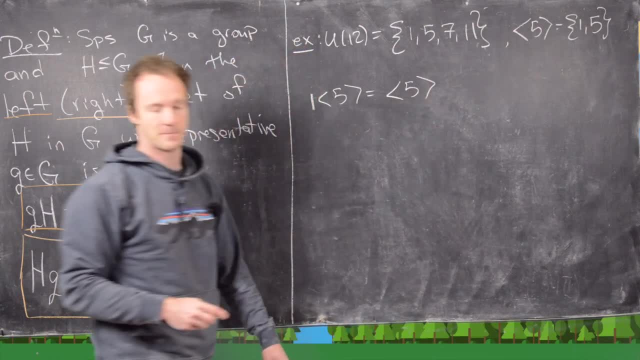 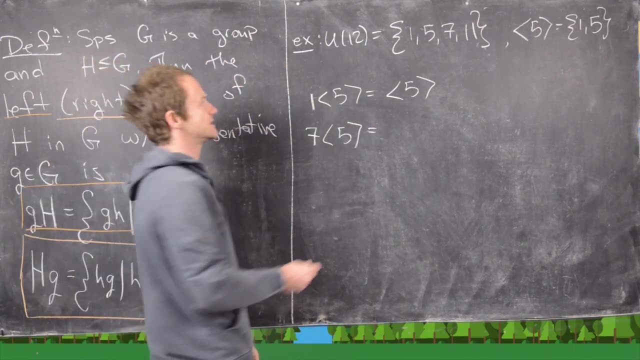 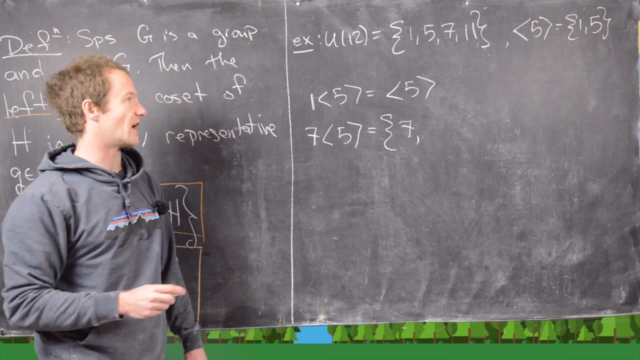 of the identity is just the subgroup itself and then let's maybe look at the coset of the element 7. So notice that's going to give us 7 and then 7 times 5 which is 35 but now notice that 35 is 1 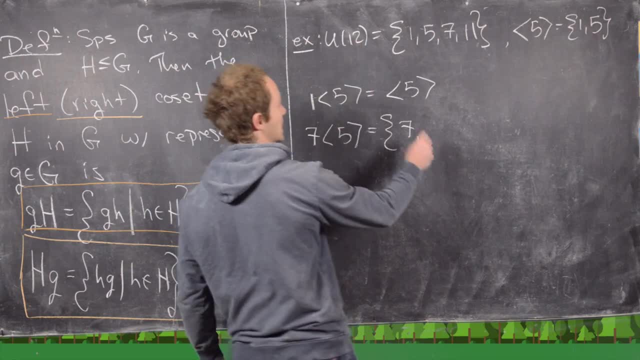 less than 36 which means it's negative 1 mod 12 which is the same thing as 11 mod 12. Okay great. 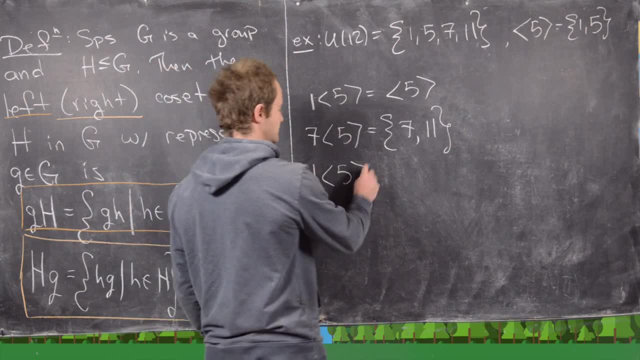 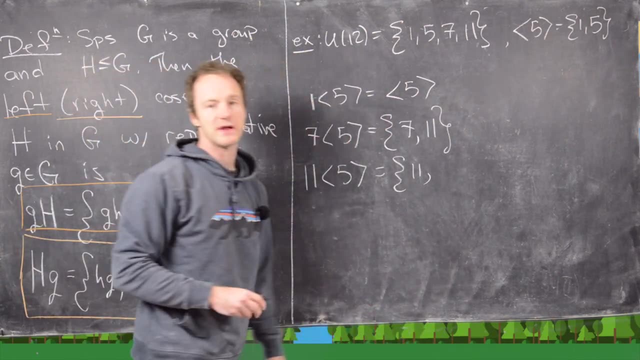 Now let's maybe look at the coset of the identity which is just the subgroup itself and then let's maybe look at the coset for 11. So notice that's going to give us 11 and then 5 times 11 which will 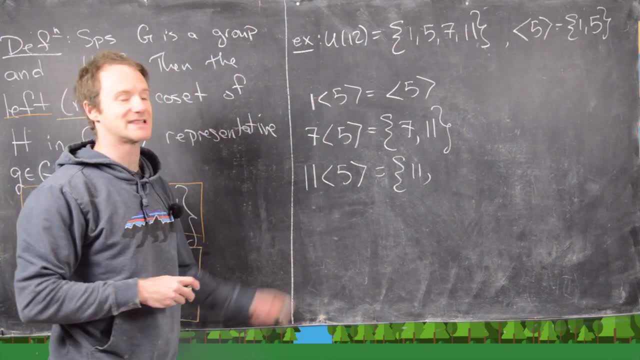 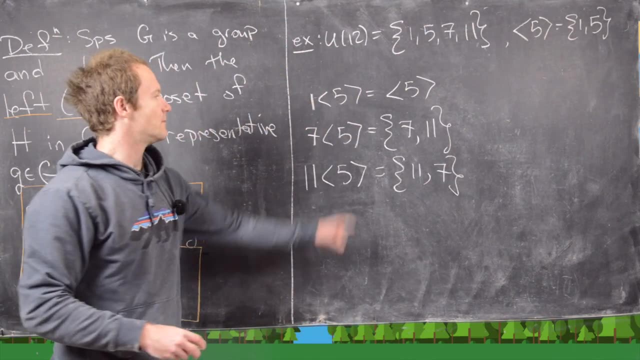 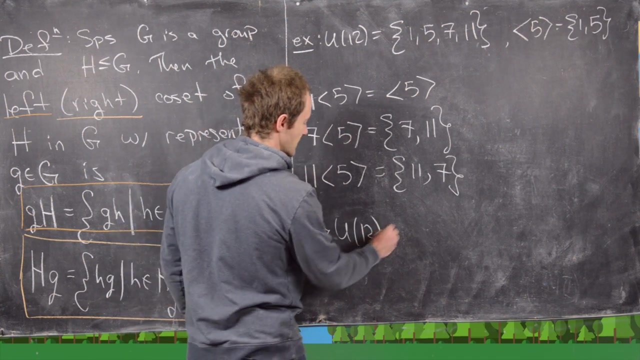 be 55 but now 55 is 7 more than 48 so that means that 55 is 7 mod 12. But now notice between 1 5 and 7 and 11 we have achieved the whole group so we can see here that u12 breaks down as we have seen before as we have achieved the whole group. So now let's look at the coset for 11. So notice that 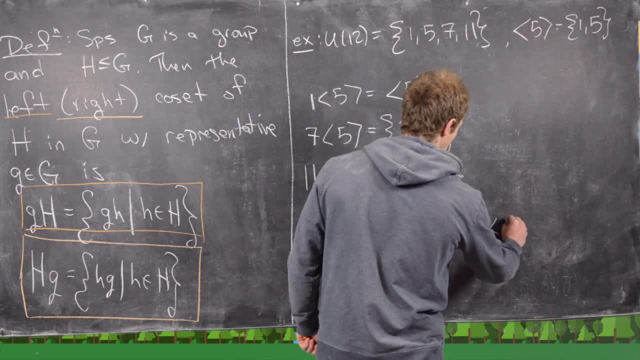 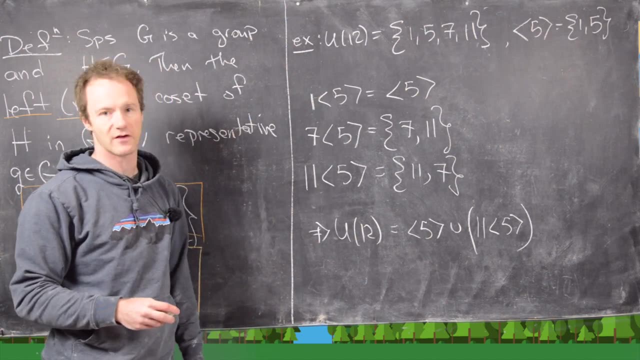 has the cyclic subgroup generated by 5 and then the coset of that cyclic subgroup with maybe representative 11 or 7. We could use either one. Okay two more examples. Okay so for our next 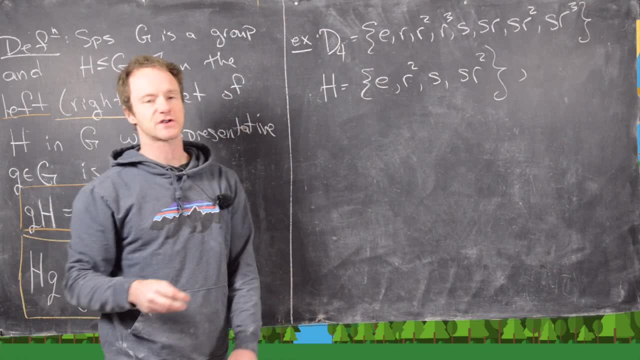 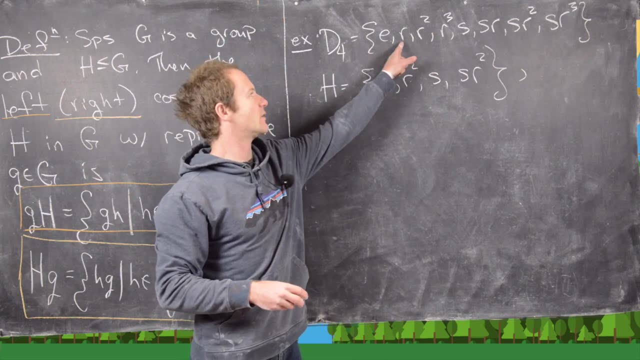 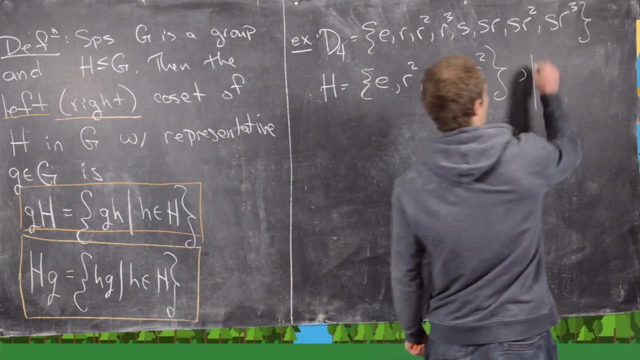 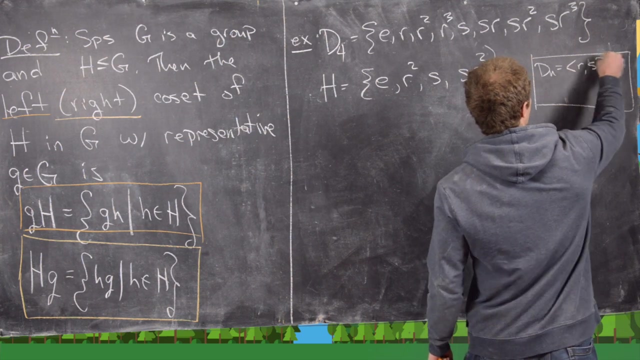 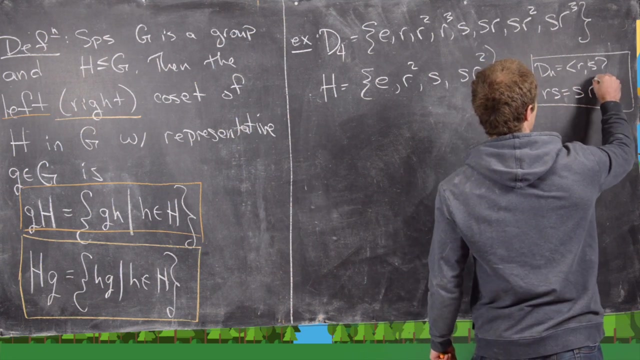 example I want to look at the dihedral group d4. So those are all symmetries of the square. So here we have four rotations. The identity which is doing nothing. Then we have 90 degrees, 180, 270 and then we have four reflections. And then let's just recall our rule for the dihedral group that dn is generated by r and s and then we have these rules that r times s is the same thing as s times r to the n minus 1. Great. So now I 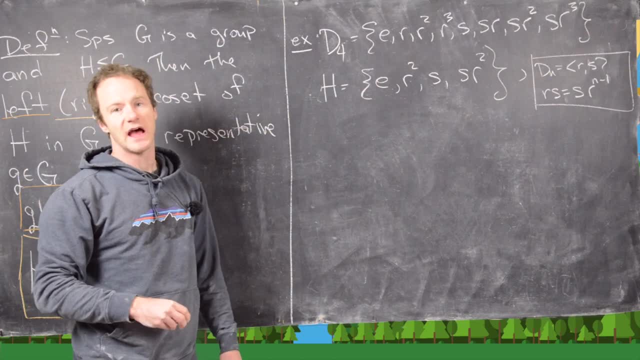 claim that this set h is actually a subgroup and we can see that pretty easily. Notice that every element in 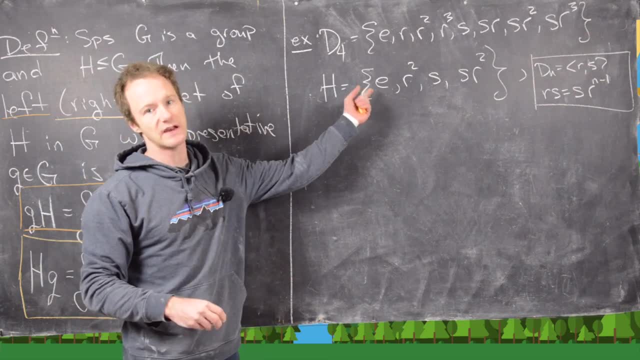 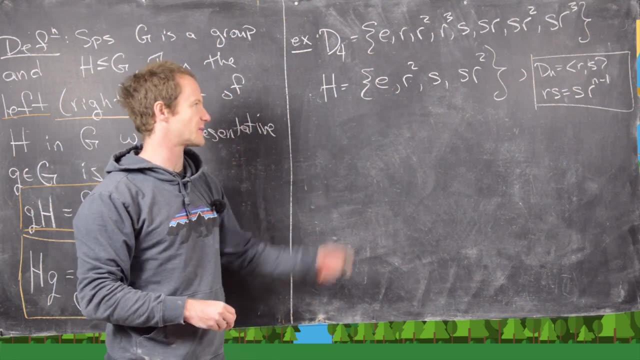 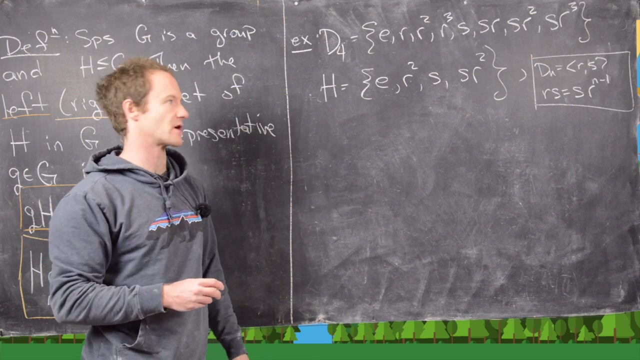 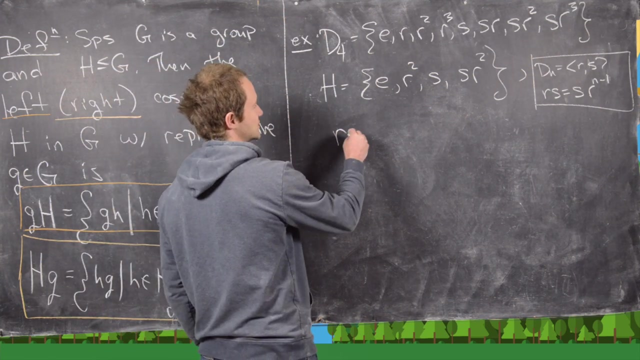 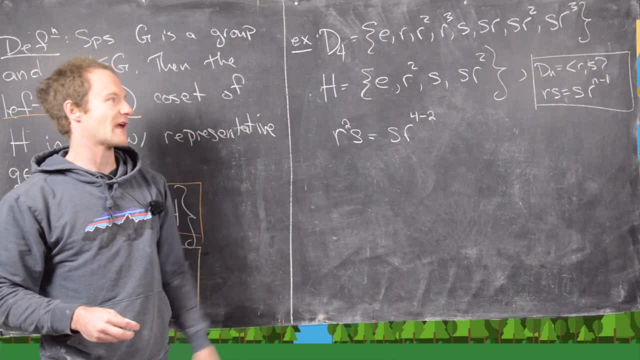 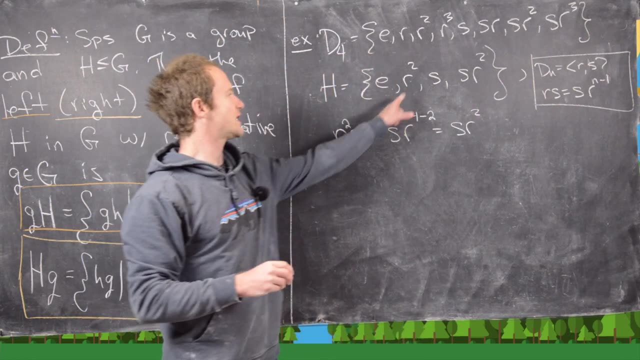 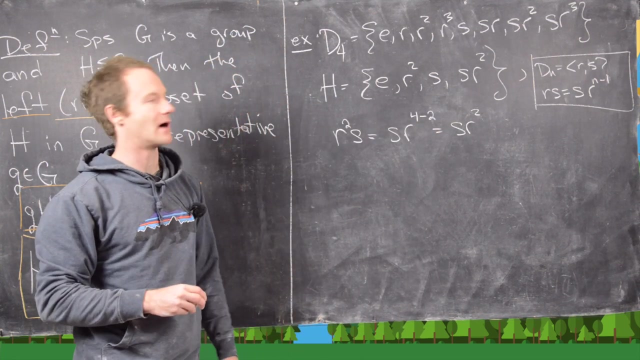 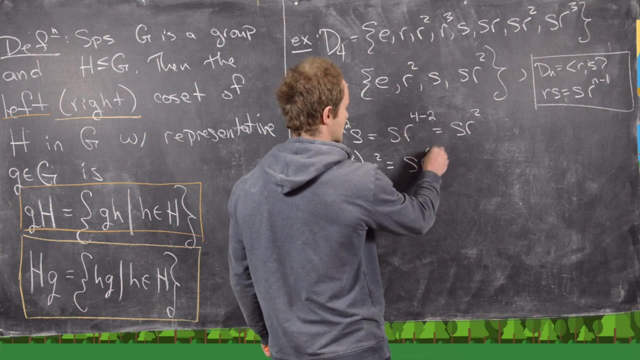 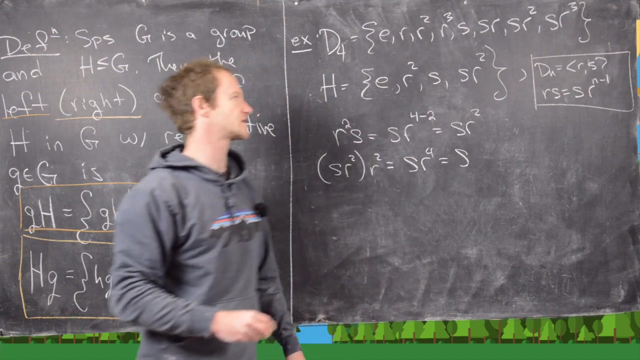 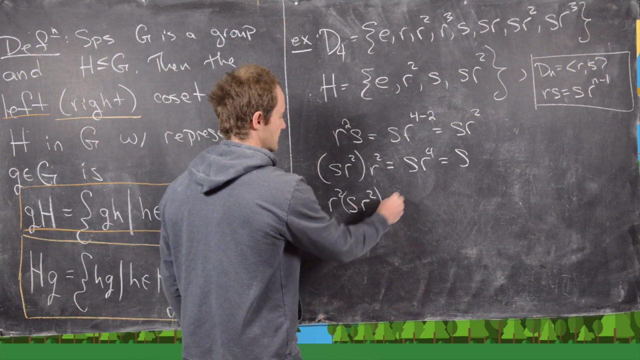 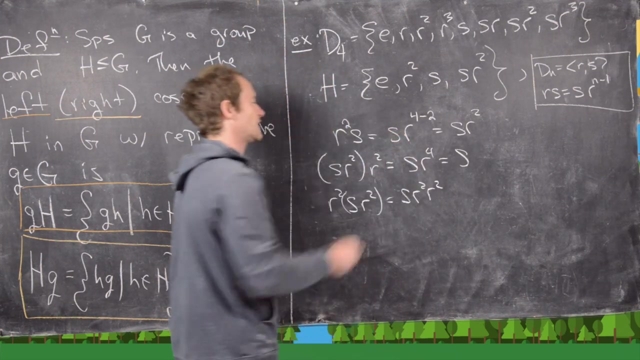 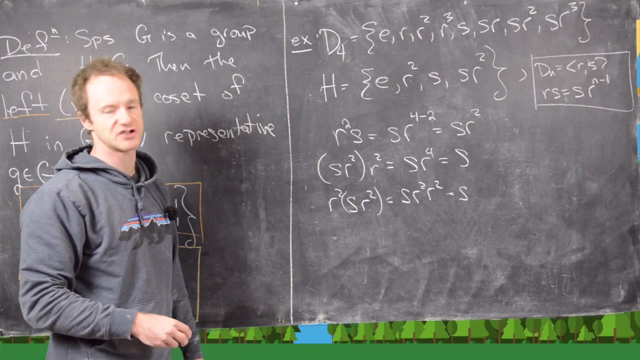 same thing as s r squared s. So that means we can multiply r squared and s together in any order and we'll get this s r squared term no problem. Now let's notice that s r squared times r squared is going to be s times r to the fourth which is s times the identity which is just s which means we can sr squared and r squared and get back in the group and then also we can do r squared times sr squared and do the same thing so we can commute this r squared past this s but you know notice that doesn't do anything just like it didn't appear and then we get r to the fourth so that gives us s and then I think there's maybe one or two more multiplications to check but I'll let 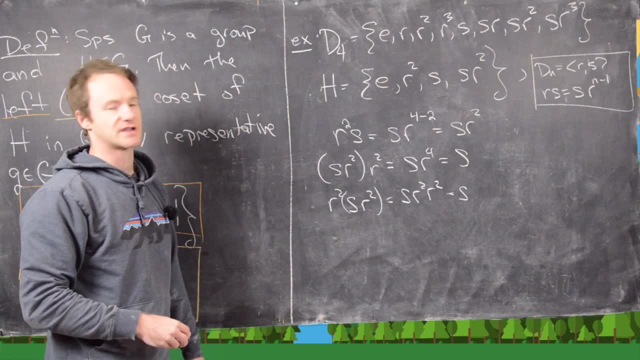 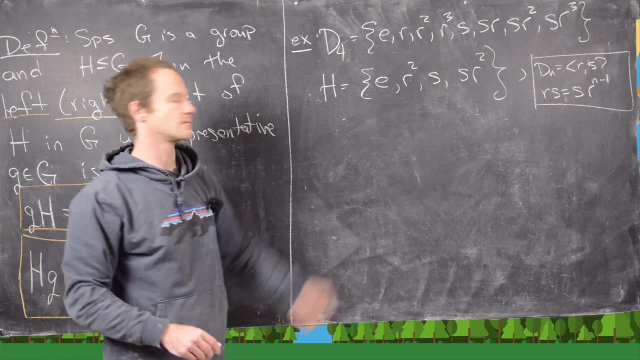 you guys check those it's pretty easy exercise okay so now that we know that this is a subgroup let's find its cosets but I'll erase this little calculation first okay so let's look at the cosets of this subgroup so if you 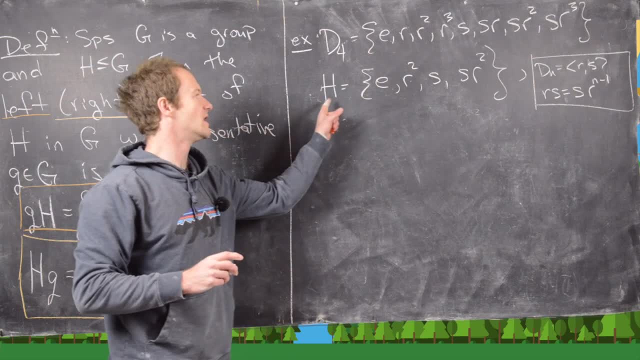 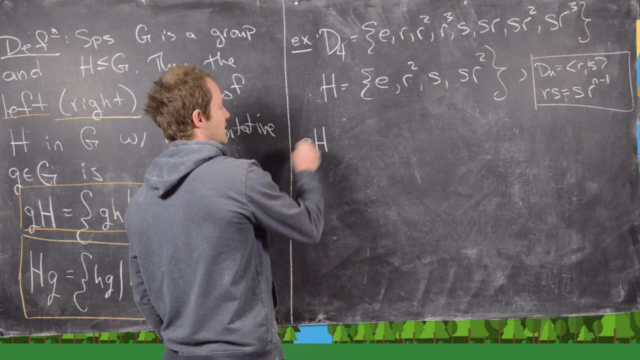 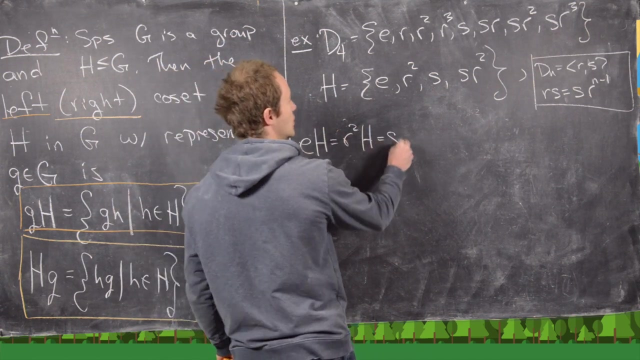 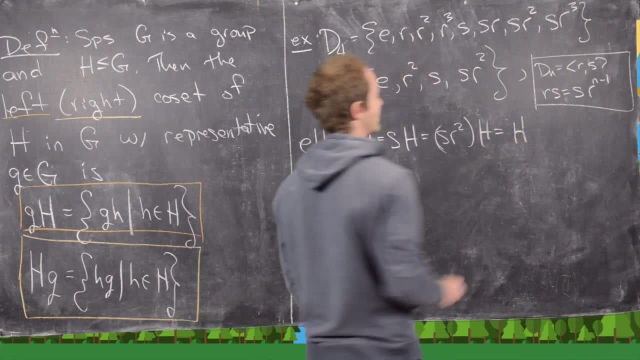 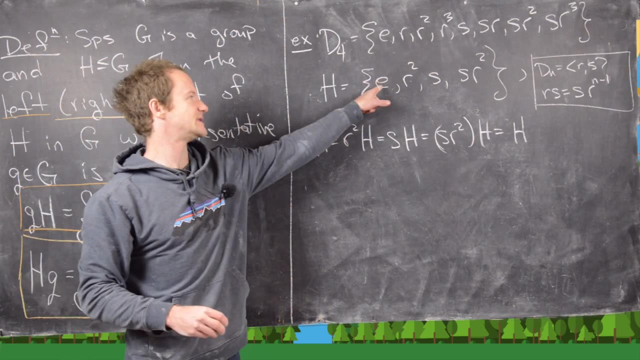 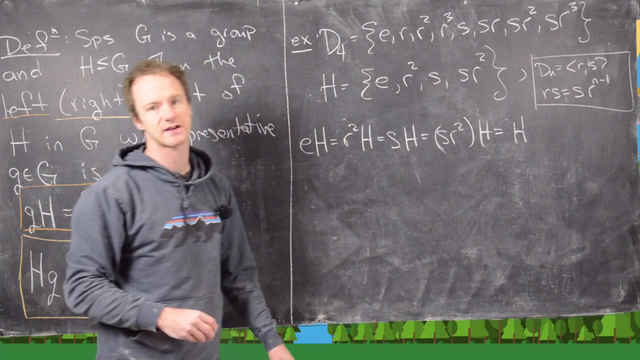 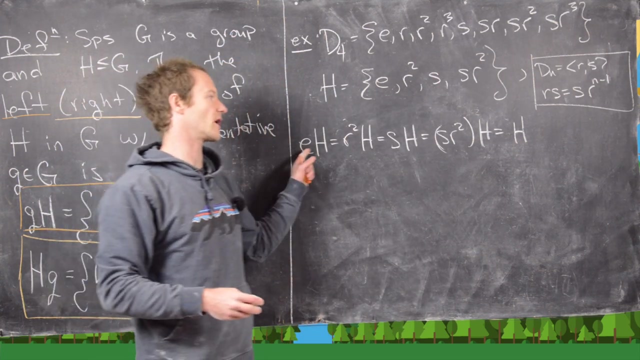 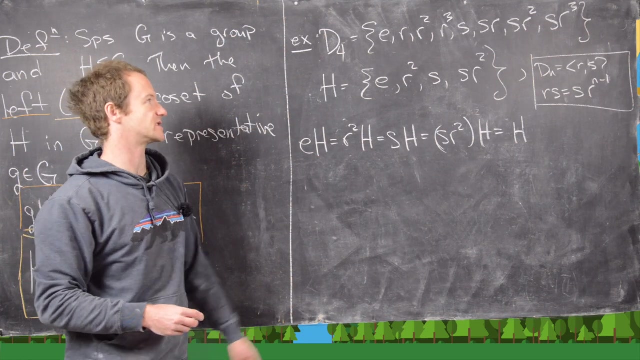 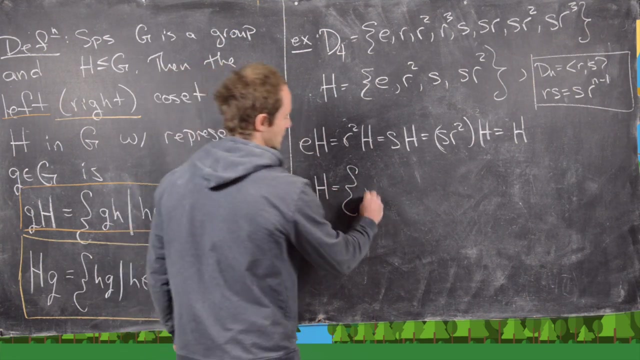 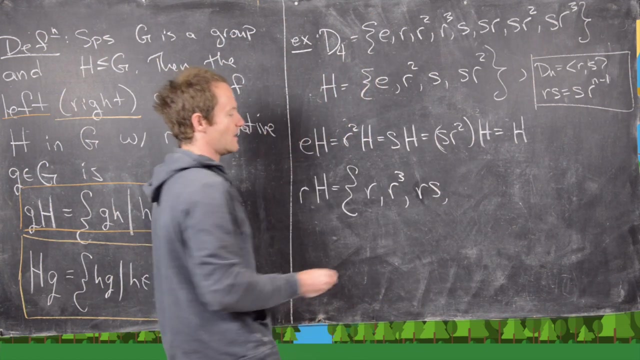 thing as SR squared which is the same thing as just having the group itself and you can see that pretty easily just by calculation so if we talk R squared times the identity we get R squared R squared times R squared we get the identity R squared times s we get SR squared like we had seen before and then R squared times SR squared we get just s as we had also seen before and then all of those are going to follow similarly so we might as well take something that is outside of this subgroup so maybe this rotation by 90 degrees so we have R times H so notice that's going to give us R R cubed so that's for these first two we'll have R times s and then finally we'll have RSR squared but 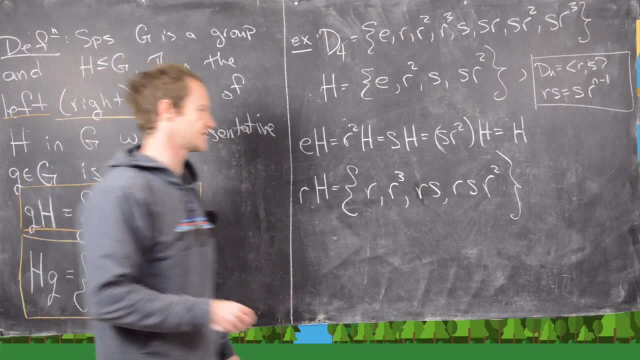 let's rewrite that so that it's in like the canonical form for these and notice 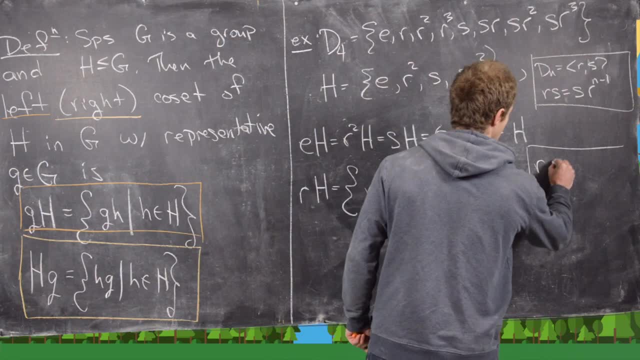 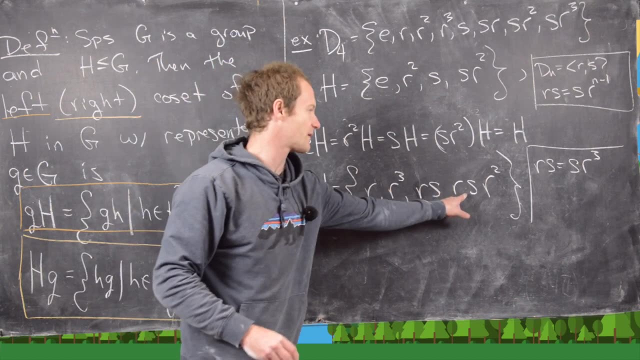 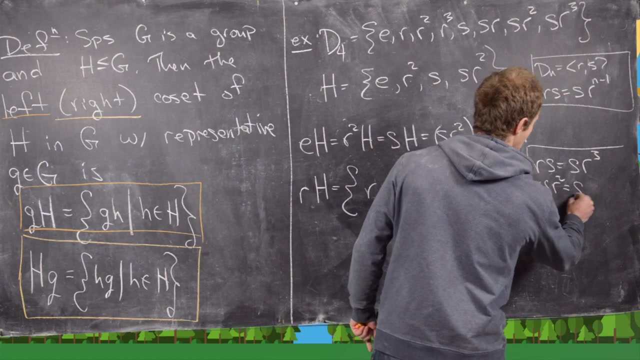 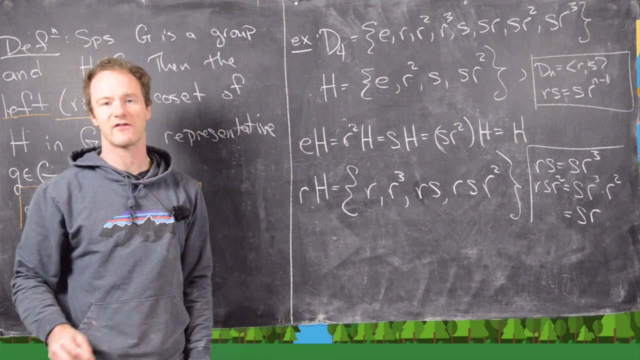 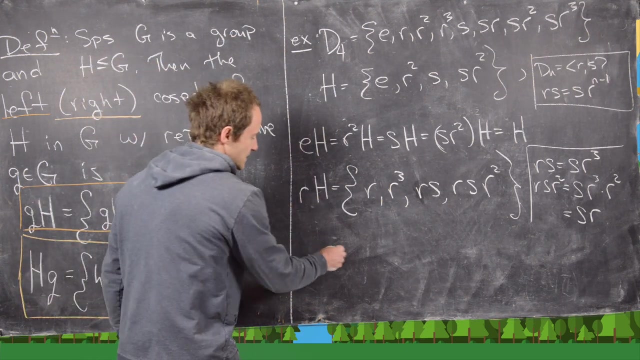 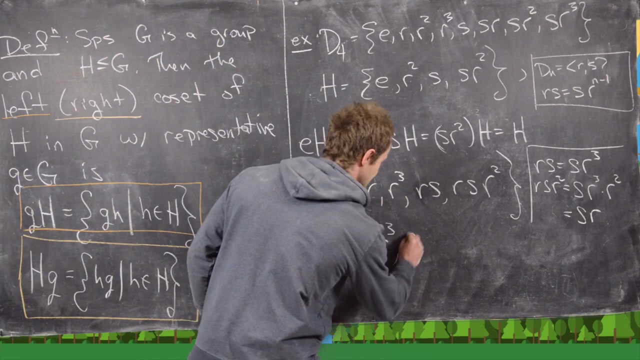 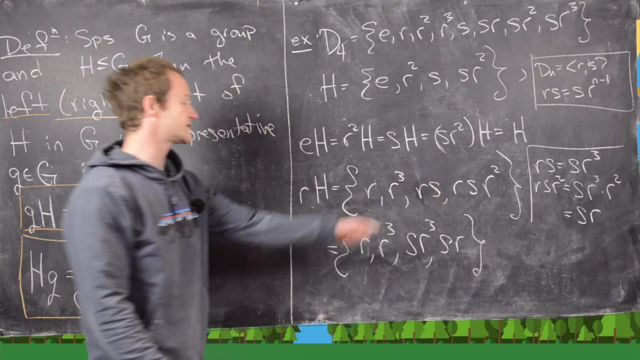 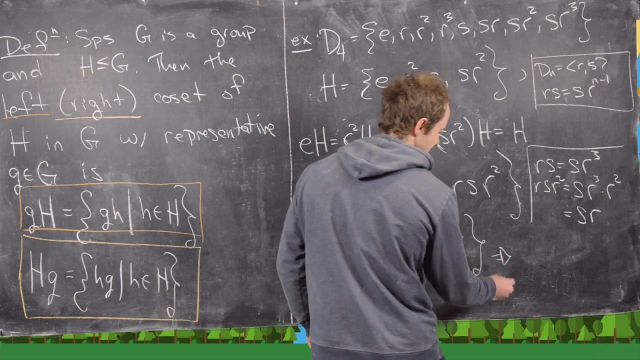 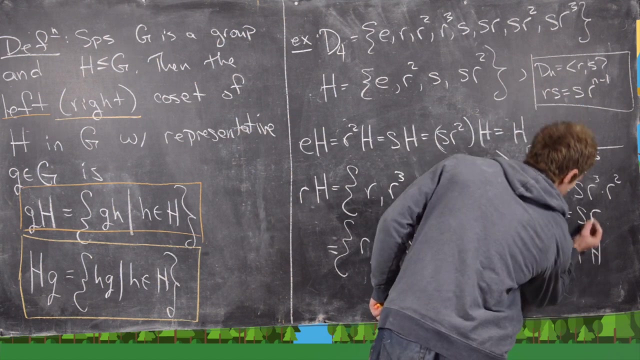 we can do that pretty easily using this rule up here so we know that all right so RS is the same thing as SR cubed in d4 and so we can apply that here and we can apply that here and when we apply it here we'll have RSR squared is the same thing as SR cubed times R squared which is the same thing as SR because there we have R to the fifth which is the same thing as R to the first given that R to the fourth power is the identity okay so all in all that says R R cubed so we've got those two rotations and then we have this which is SR cubed and then we have this one which we calculated down just to be SR and notice those are all of the elements of D4 that are not in the subgroup and so what that tells us is that D4 can be written as this subgroup unioned with this coset which is RH okay good so I'll clean up the board and then we'll do 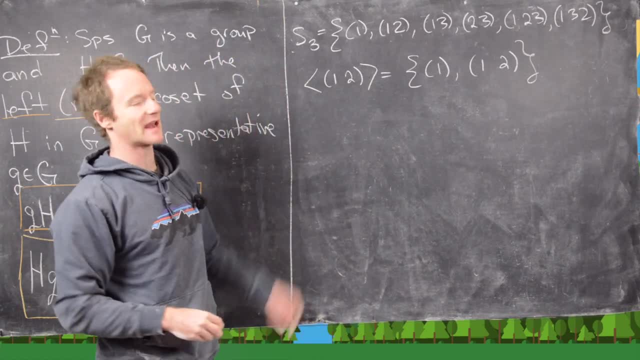 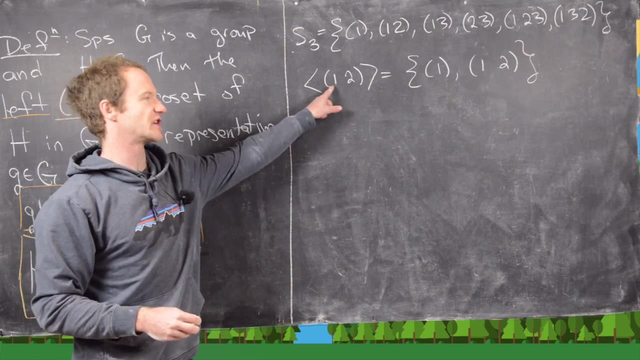 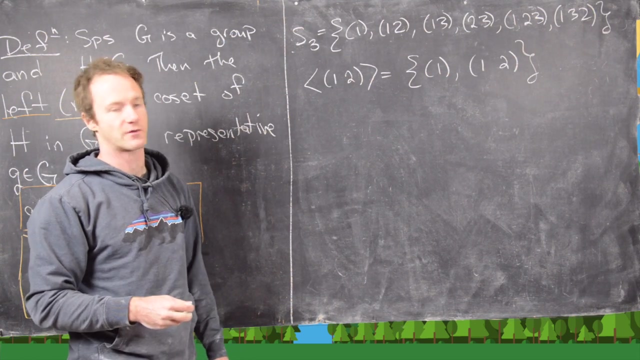 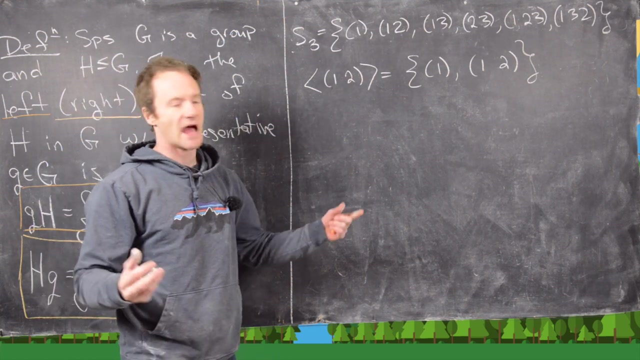 one more example okay so for our last example we'll look at S3 so the symmetric group on three letters and we'll look at this cyclic subgroup generated by the transposition 1 2 so here we're using cycle notation which hopefully you've seen before I've got a video on it if you need to refresh okay so the transposition 1 2 is obviously its own inverse as you can see if you compose this with itself 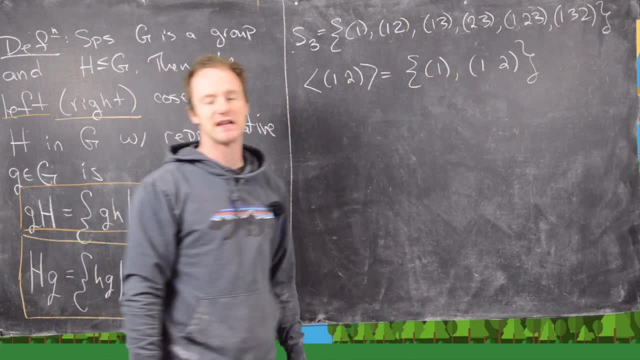 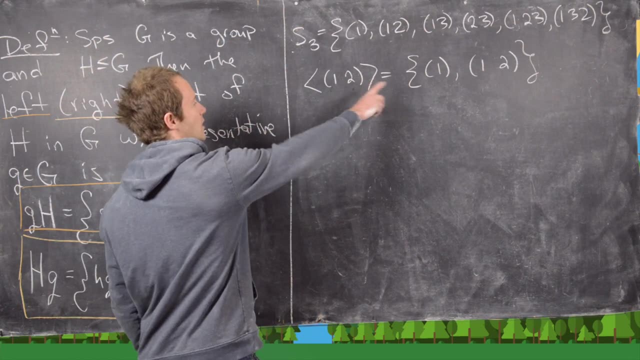 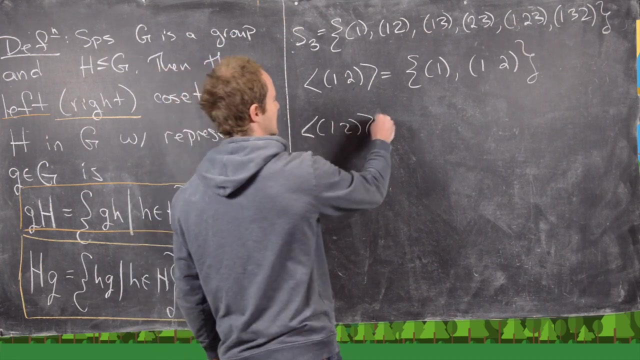 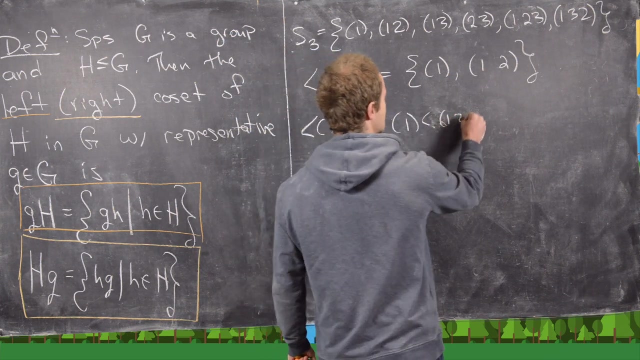 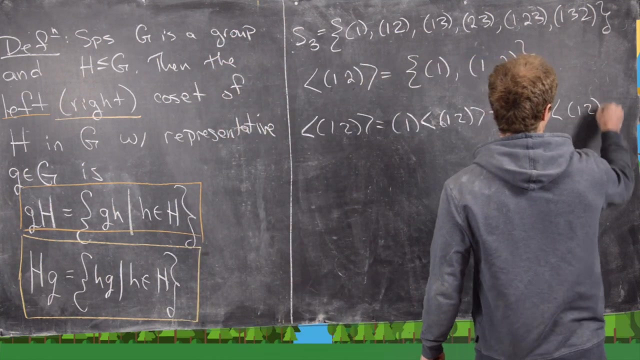 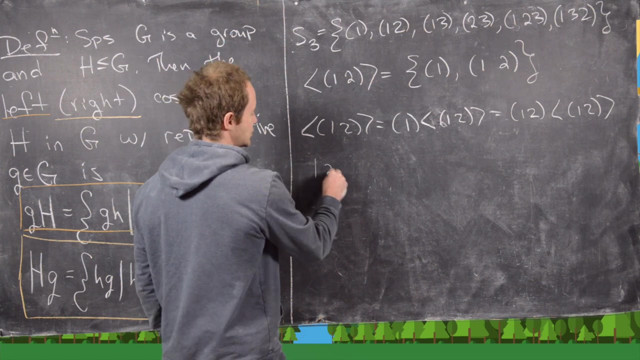 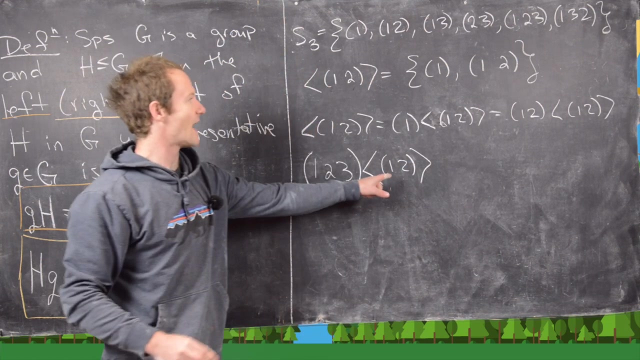 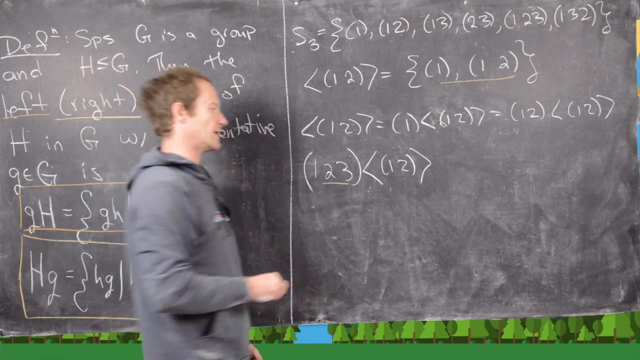 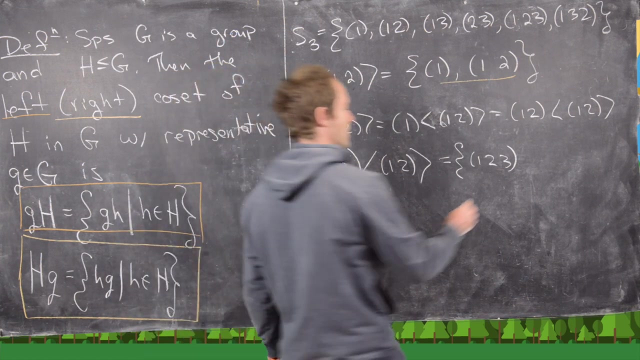 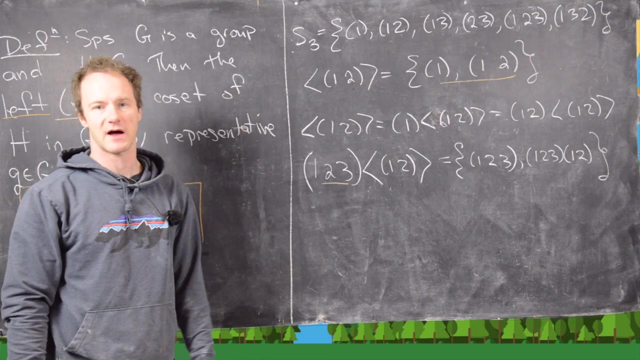 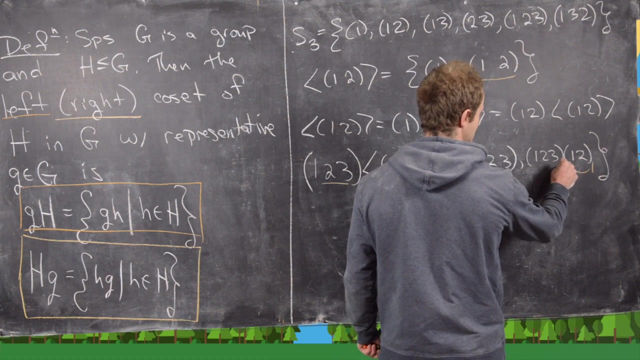 you get the identity so that means this subgroup is just the identity and that transposition 1 2 so let's go ahead and look at some cosets so as before we don't really need to look at the cosets with any of the elements from here because we can see that those are just going to give us that cyclic subgroup back so that means if we take the coset representative that's going to be the cyclic subgroup that we're going to use as an element so we're going to look at the coset representative and we're going to look at the coset representative the identity I just get the cyclic subgroup and then also if I take the coset representative which is that transposition I also just get that cyclic subgroup okay great so now let's take maybe 1 2 3 let's take that to be our coset representative so that means that we need to multiply everything in this cyclic subgroup by this 3 cycle 1 2 3 okay so that's going to give us 1 2 3 that's what we get when we multiply it by the identity and then here we get 1 2 3 times 1 2 that's what we get when we multiply it by that so now let's see what we get here so 1 gets sent through this first transposition to 2 and then through the second one to 3 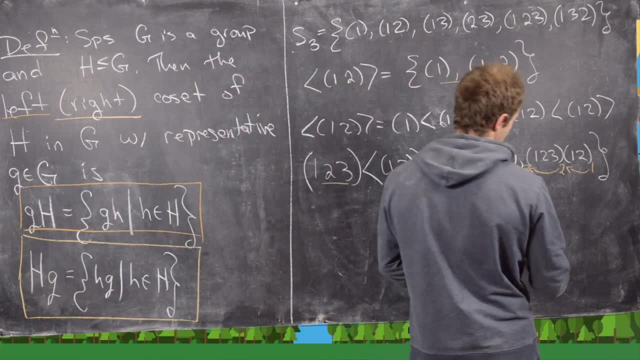 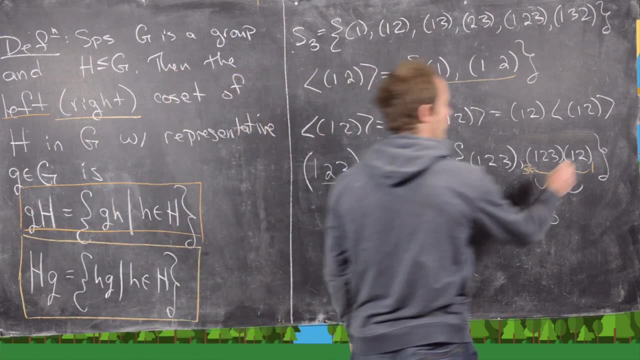 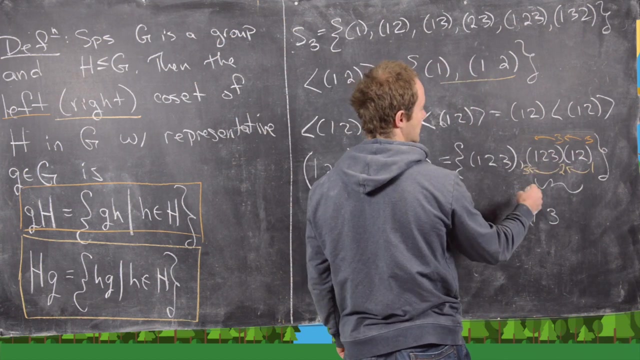 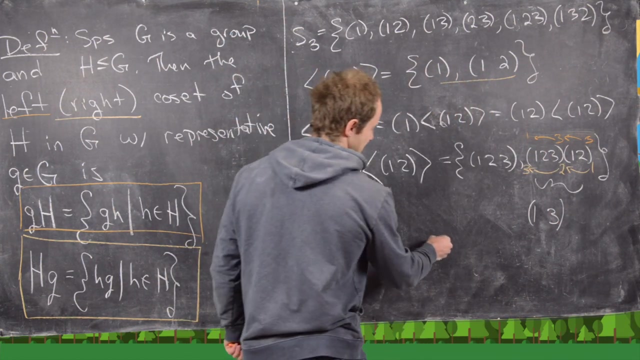 great and then that means we know that this thing starts off like one three great and then three is unchanged by this rightmost permutation and then by the first one it gets sent to one which means we can close this up which tells us that inside of this coset we have the element one two three 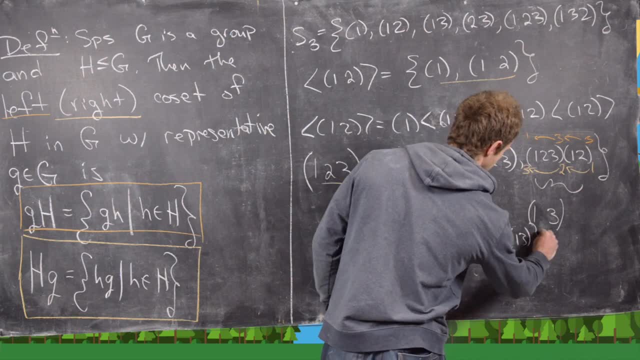 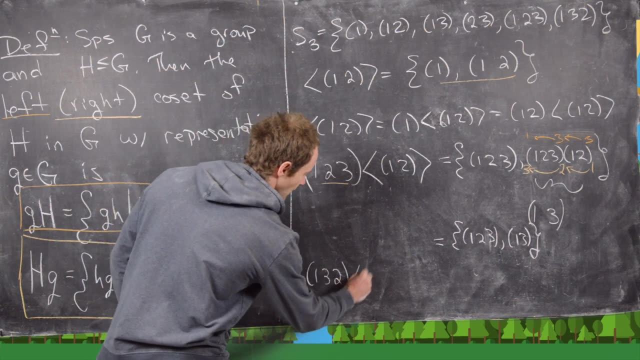 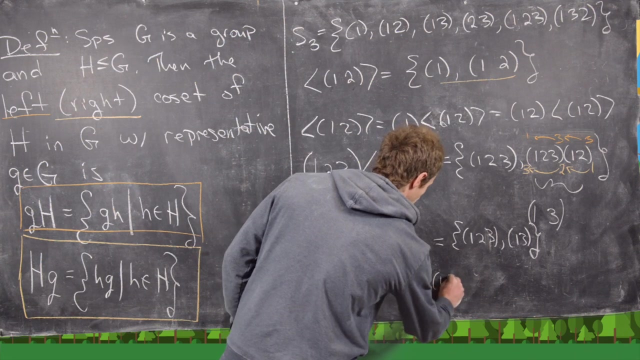 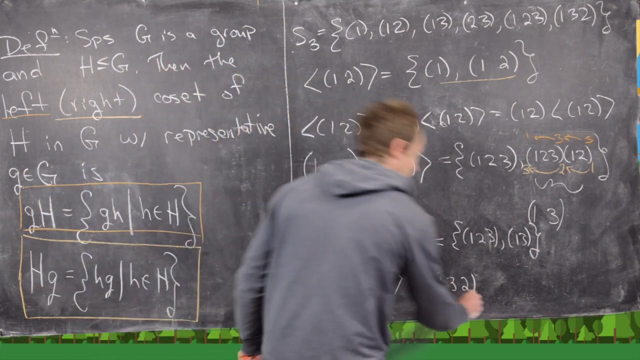 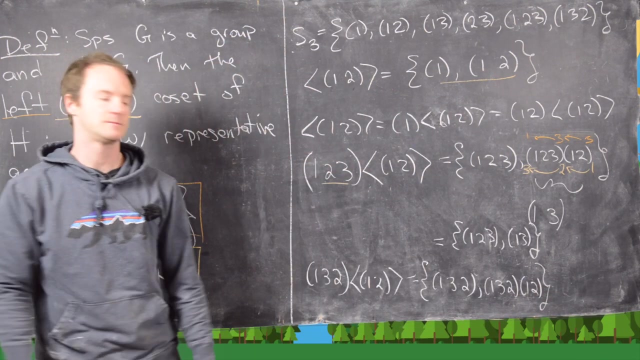 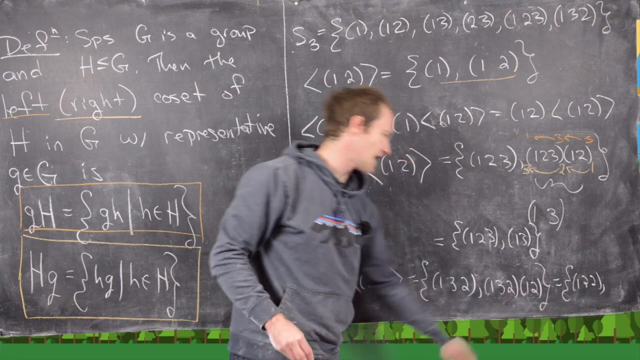 and then the two cycle one three great and now let's check one more so let's do one three two on this one two cyclic subgroup and notice that's going to give us one three two that's what we get when we multiply one three two by the identity and then we need to multiply one three two by our generator which is one three two by the identity and then we need to multiply one three two great and then this is going to give us one three two and then you can check here